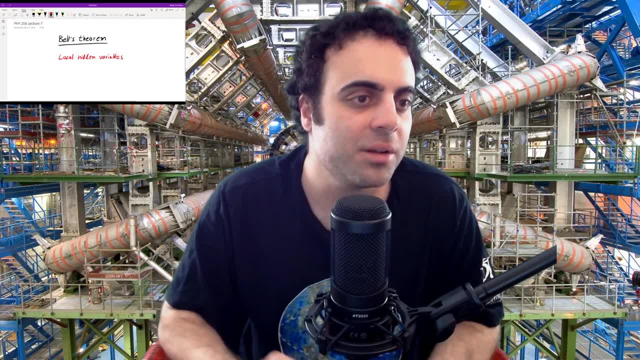 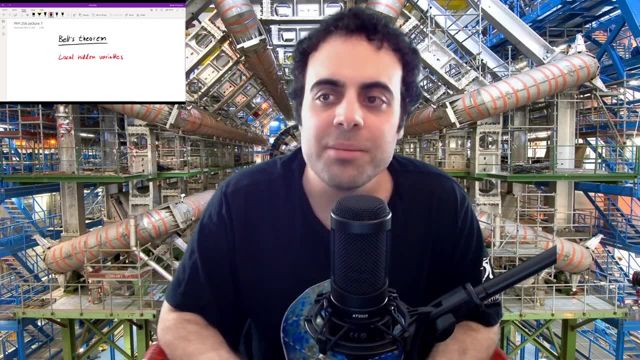 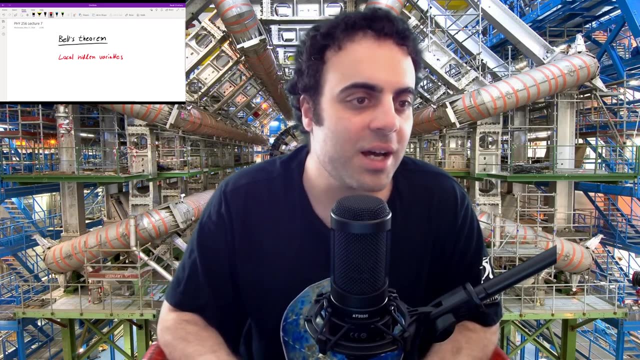 other note and then I place the notes in the envelope and I seal the envelopes and then I give 1 to Alice and 1 to Bob and then Bob goes away to Alpha Centauri and he opens his envelope and if he sees 0 then he knows that Alice. 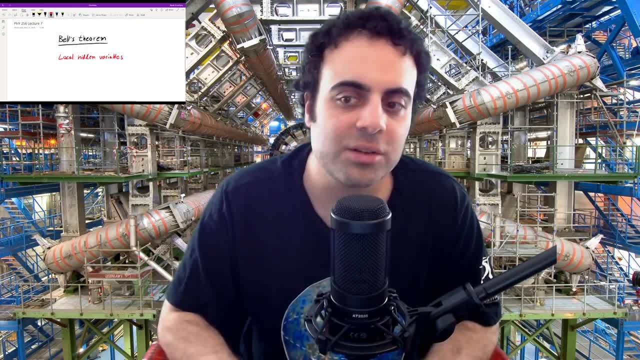 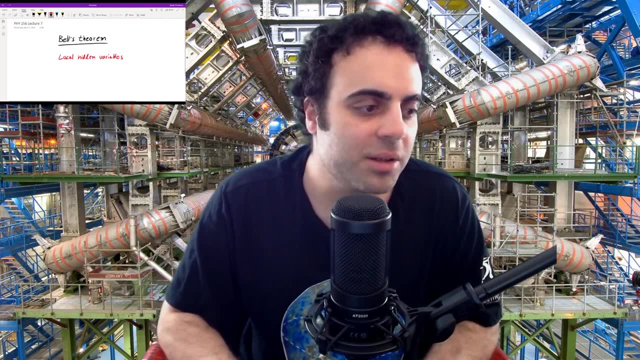 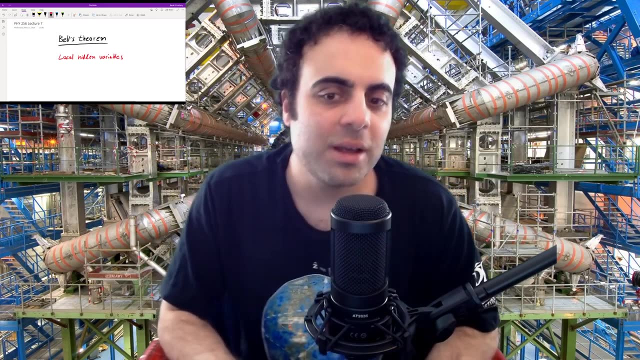 has 1 in her envelope, and this is just classical correlation. So I'm going to show you how to do this. So I'm going to show you how to do this. So a local hidden variable theory would be basically the same as this classical envelope scenario. The envelope always had the number 0 inside it and if 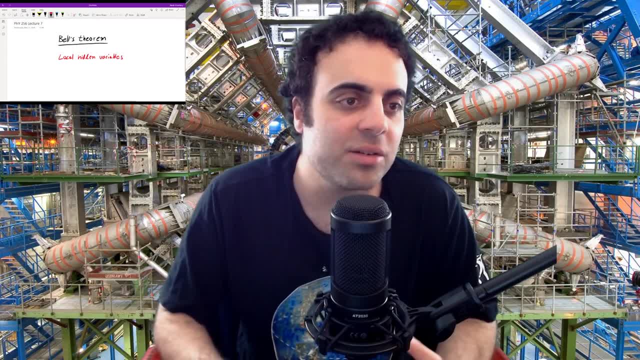 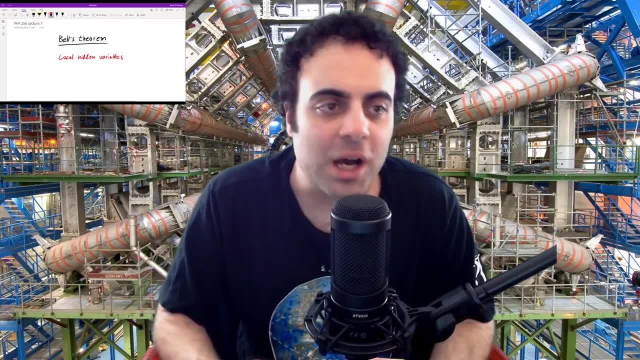 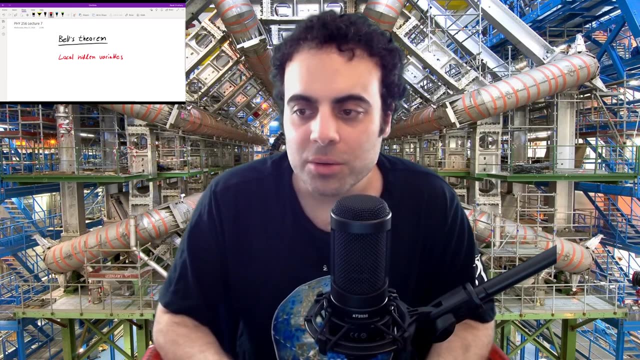 we could look into. if we could look inside the envelope at the hidden variable that is inside the envelope, without opening it and doing the measurement, we would have been able to make a deterministic prediction. So in this sense, local hidden variable theories have classical correlations and Bell's theorem that we will now prove it proves that quantum. 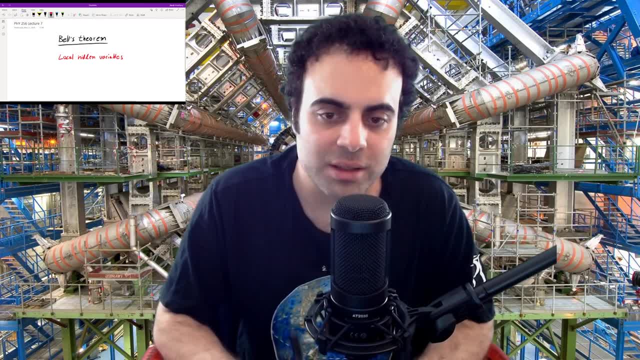 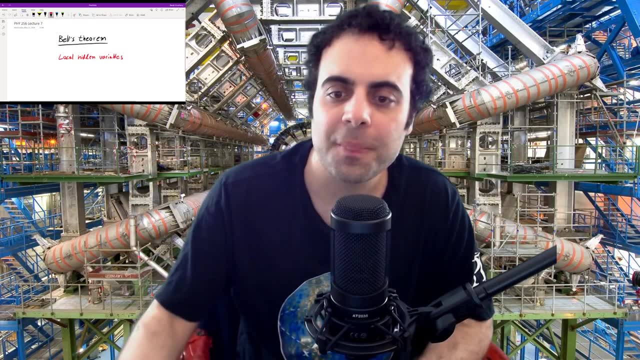 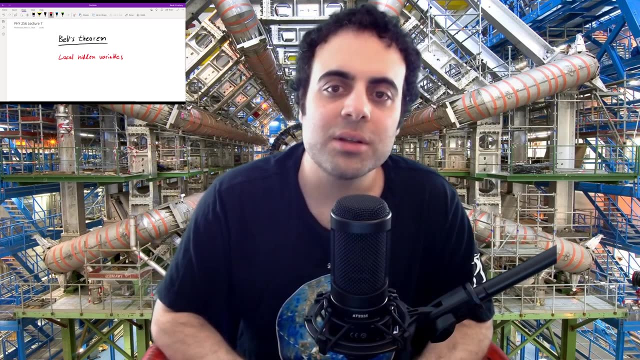 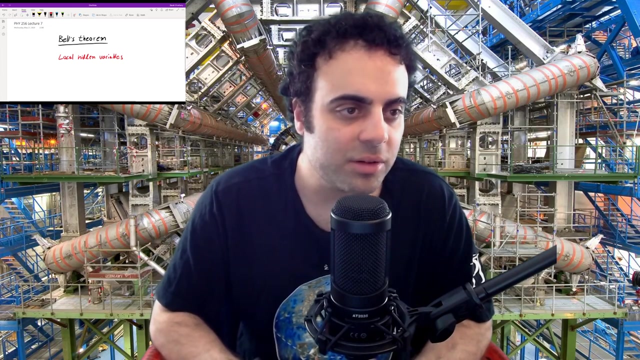 entanglement is different and, in a precise sense that we will soon discuss, stronger than classical correlation. Okay, so let's do the proof. So let's consider the following experiment. I prepare two systems, let's say qubits, and I give 1 to Alice. 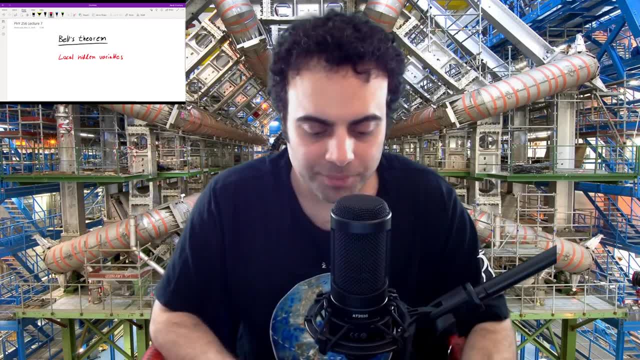 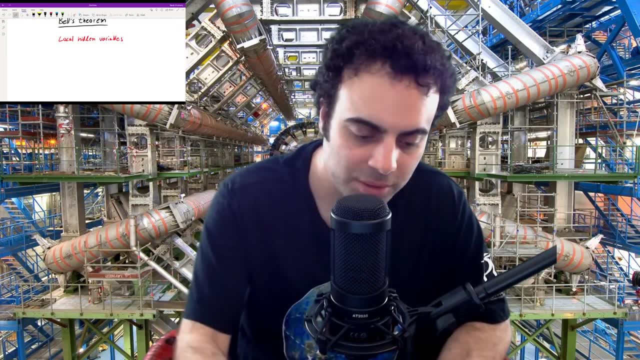 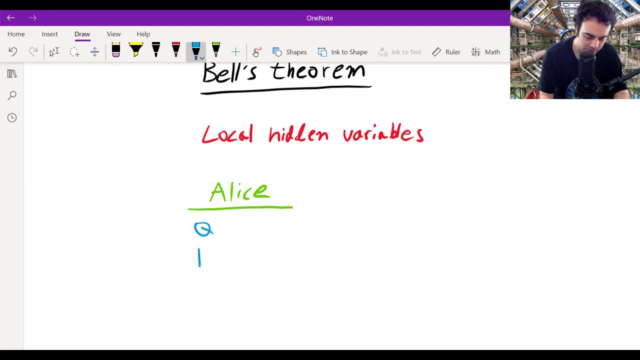 and another to Bob. Now Alice can measure 1 of 2 different physical observables of her qubit, and these observables are going to be Q and R And each of them can have either plus 1 or minus 1. as a result, 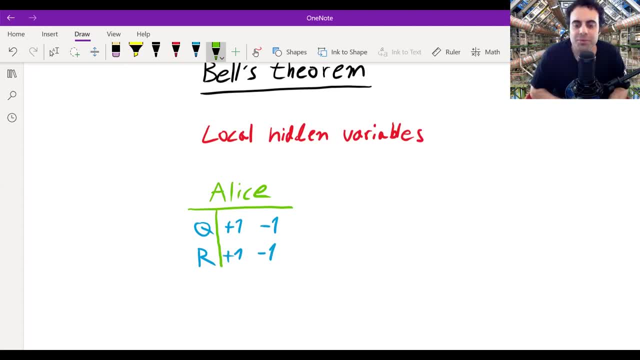 Now Bob can measure 1 of 2 different physical observables of his qubits. Let's call them S and T, and again, each one of them can be either plus 1 or minus 1.. Now these Q R, S and T are just any observables that have one of two one. 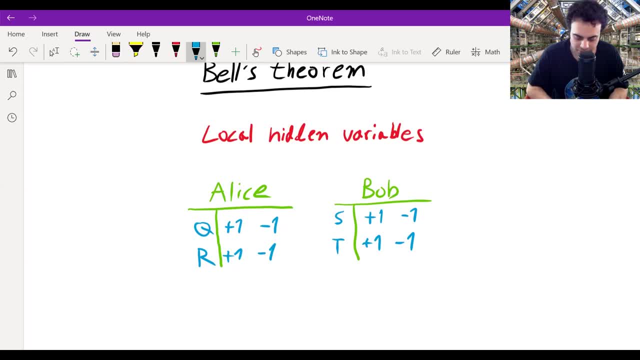 of two values. But of course we already know that the Pauli matrices, for example, have the eigenvalues plus 1 and minus 1, so it would make sense to choose the Pauli matrices or some linear combination of the Pauli matrices in order to make the Pauli matrices as these observables. and this is exactly what 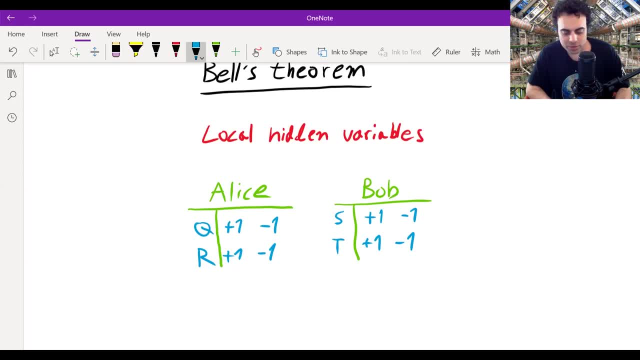 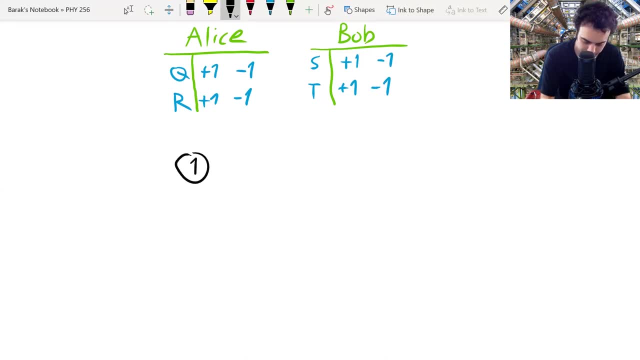 we're going to do. And now we make two crucial assumptions. Assumption number one is locality. So this assumption: we assume that both Alice and Bob measure their qubits at the same time and at the same time they measure their qubits at the same time. 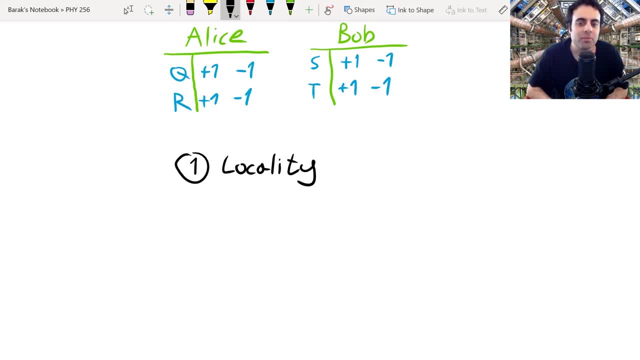 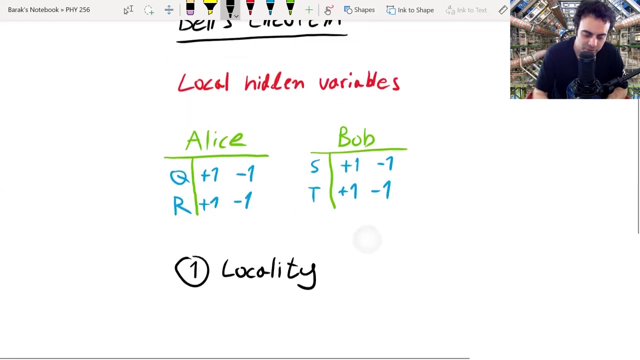 In different places, so that the measurements cannot possibly disturb or influence each other without sending information faster than light, And this ensures that the predicted probabilities for Alice and Bob's measurements are completely independent of each other. So this condition is the one that corresponds to the local in local hidden variable theory. 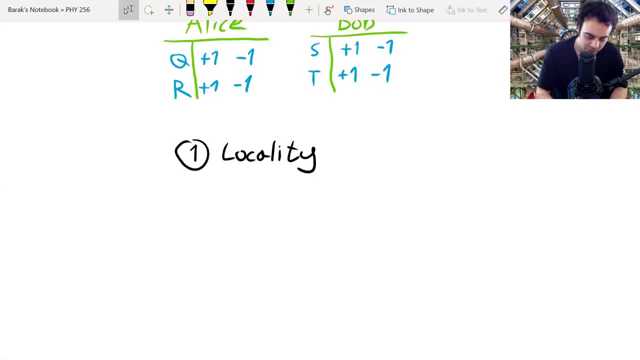 The second condition is the condition of realism, and this assumption is that the values of the physical observables Q, R, S and T exist independently of observation. So they have certain definite values which are already determined before any measurement took place, Just like in the envelope scenario. So Q, for example, has been plus one all along. 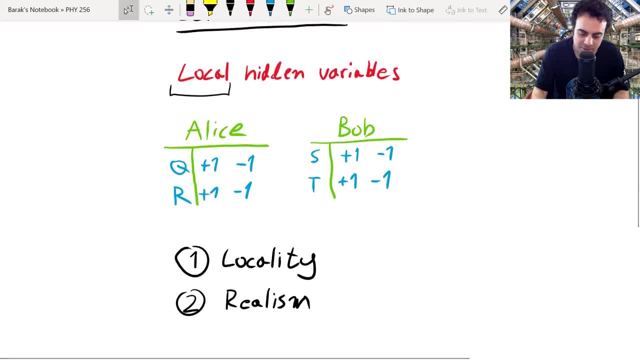 And this is exactly where the hidden variables come from. The hidden variables encode the information about what are the actual values of these observables that have already existed before I measured. Now, then, what Đâyтery rules will do is to Concern, not only answer, the particular horse's. 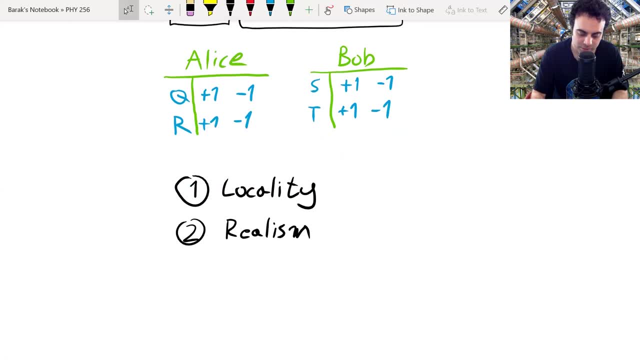 говорables, but also to be able tokäadyiz gén cheat. a Yakitori formula about the number of times paper iskurk and the number of times paper is 不能 inculcated and the number of times box front and back count as n и shape. 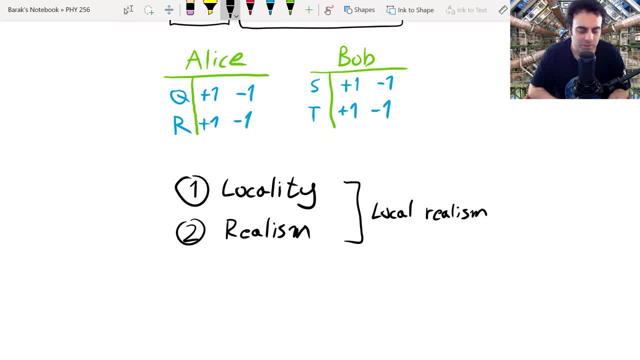 The questions that need to be answered will not only depict how often the index y will be discernedств promote the number of times the index y will be control, but also how often it will be broken down by the square root. Besides this, we can write coming together the integral x, y, z and z. This form must never be consistent with the end cargo in order not to give either value to the space. So for key violet face values, value is required as a Stern in a genom, one less value to be happening in the set of expressions. 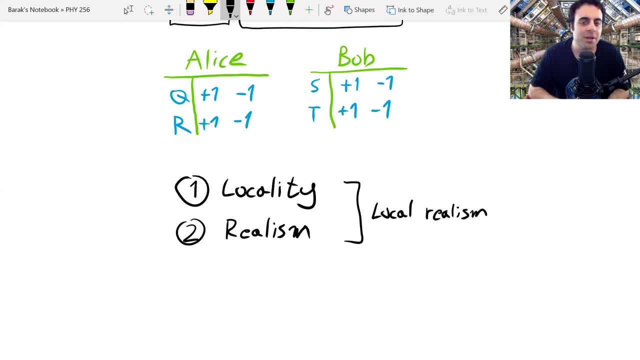 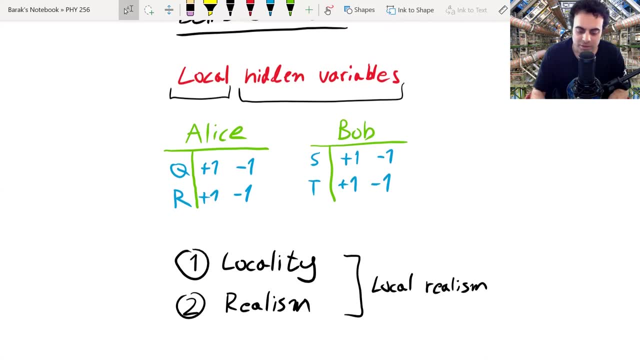 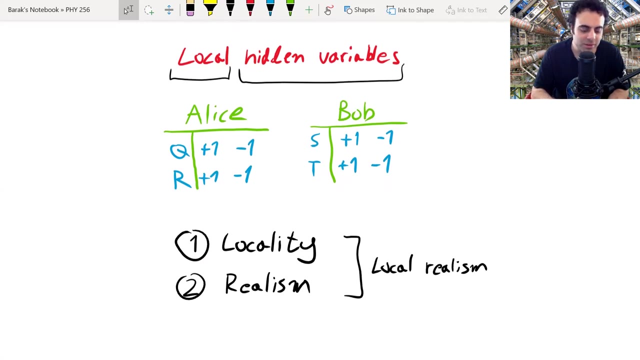 realism. Local hidden variable theories also satisfy this principle. as we have seen here, There's also non-local hidden variable theories which satisfy realism, so they are still deterministic, but they don't satisfy locality, so they do in fact allow information to be. 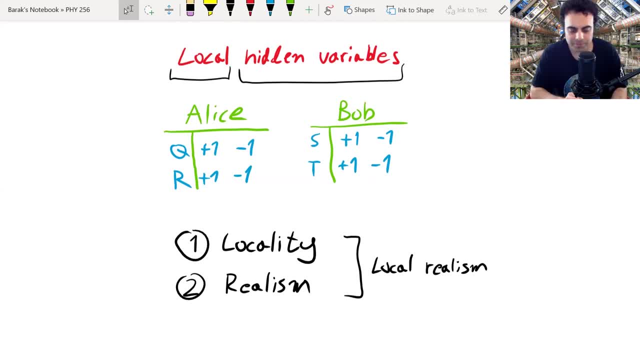 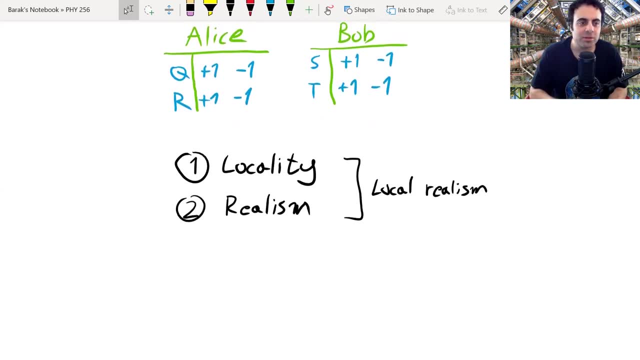 transmitted faster than light. So the proof now goes as follows: When I measure the values of q, r, s and t, we said that each one of them can be either plus one or minus one. Okay, so let's say that lowercase q, r, s and t are the values that we actually measured. 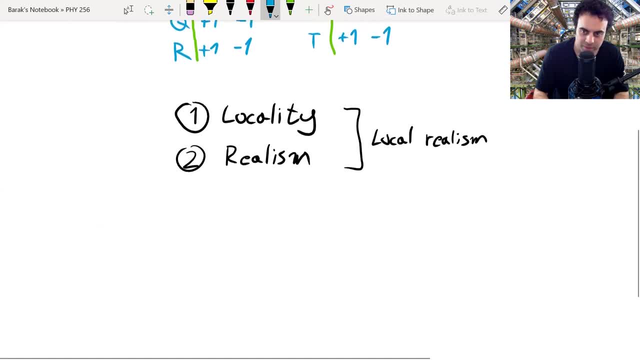 and then we can say that q, r s and t are the values that we actually measured, and then we can say that q, r s and t are the values that we actually measured. then there is this particular combination: r s plus q s plus r t minus q t. 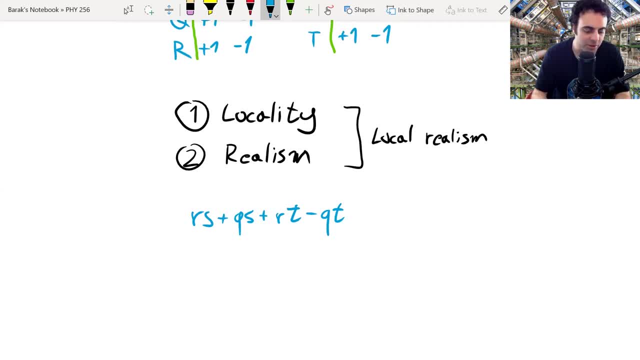 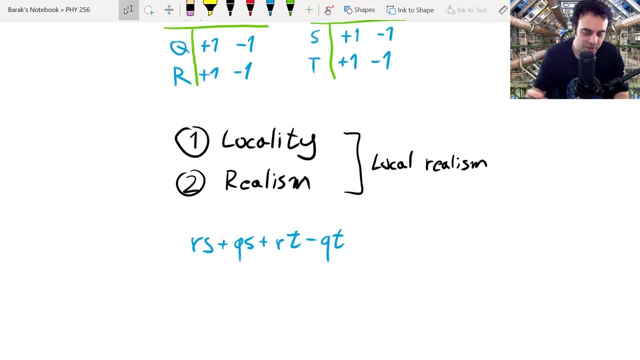 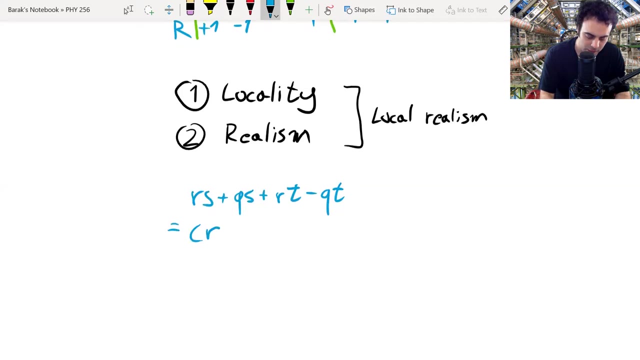 So r is the value that we measured for the observable r. so either plus or minus one s we measured for the observable s and it's either plus one or minus one, and so on. So we can write this as r plus q times s. plus r minus q times t. 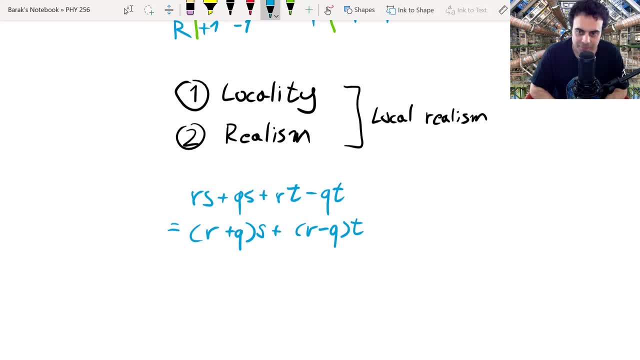 Now for this expression. notice that there's r plus q and there's r minus q, So we can write this as r plus q times s, plus r minus q times t. Since both of them can be either plus or minus one, we have exactly two cases. 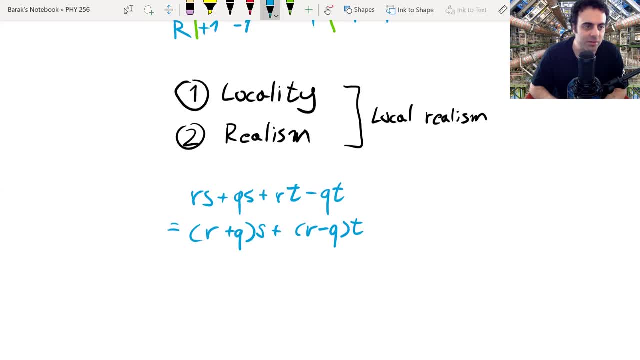 Either r and q have opposite signs. let's say r is plus one and q is minus one, or vice versa. and then r plus q is going to be zero, or they both have the same sign. so let's say r and q are both plus one or they're both minus one. 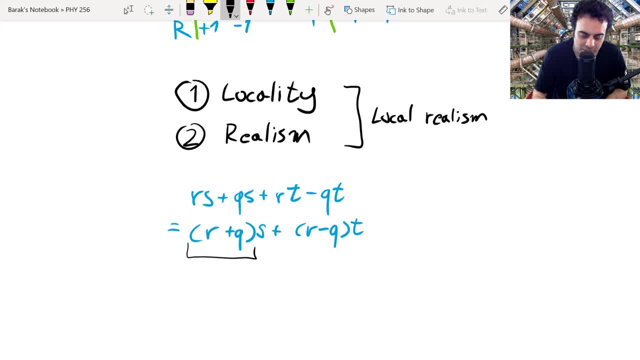 in which case we will have that R minus Q is equal to zero. So in any case, one of these two terms has to vanish and we are left with just one term. Now, in the first case, where R plus Q is equal to zero, we only have the second term left. 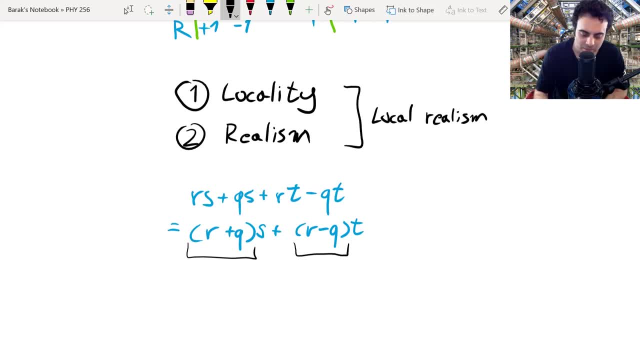 and then R minus Q is gonna be either plus 2 or minus 2, so it's plus 2. if, for example, R is plus 1 and Q is minus 1 and T is either plus 1 or minus 1, so in total this entire term is gonna be plus or minus 2.. 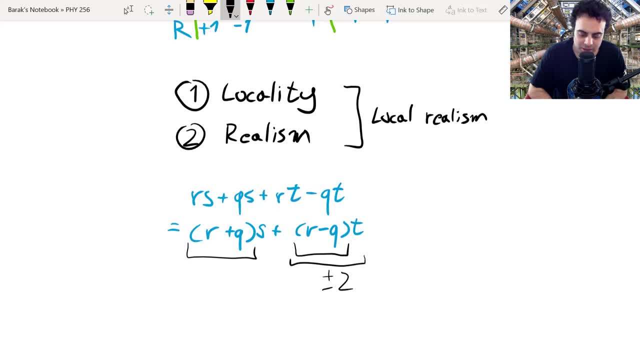 Similarly in the second case, where R and Q have the same sign, then now the second term is zero, but the first term- R plus Q, because they have the same sign- can either be plus 2 if they're both plus 1, or minus 2 if they're both minus. 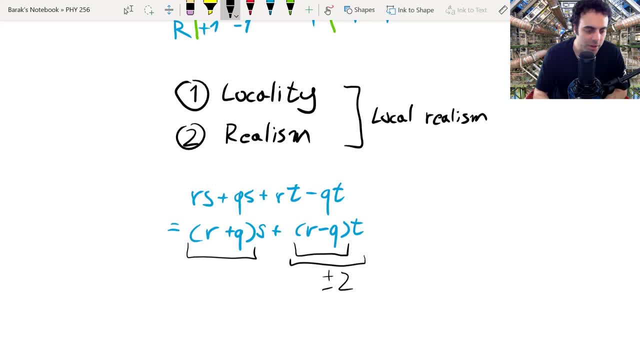 1. so plus or minus 2, and then S is plus or minus 1. so again we see that for the entire term it's plus or minus 2, and then S is plus or minus 1. so again we see that for the entire first term it can have either plus or minus 2 as its value. So in total we see. 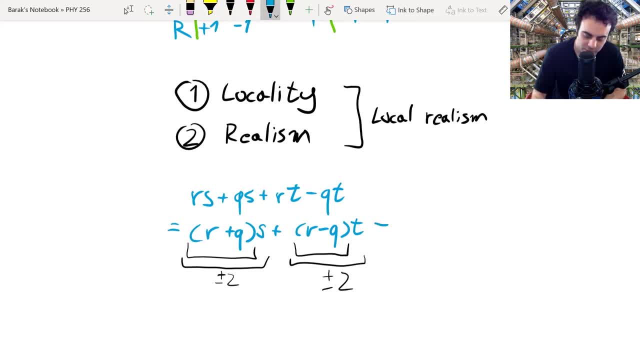 that this entire expression is equal to either plus or minus 2.. There's a question on the chat: where was the first line from? The first line is just some combination of the observables that I just I decided I'm gonna look at this particular combination: R S plus Q S plus R T minus Q T is just, it's some. 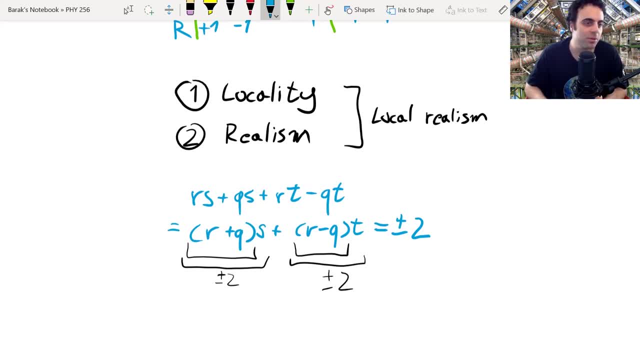 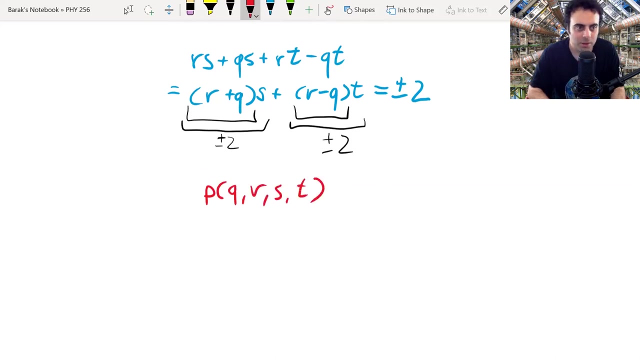 combination that turns out to either be plus or minus 2.. So now to calculate the expectation value of this expression, of course we need to assign a probability to each outcome. So there's gonna be some probability- P, of Q, R, S, T, which is gonna be the probability to measure each. 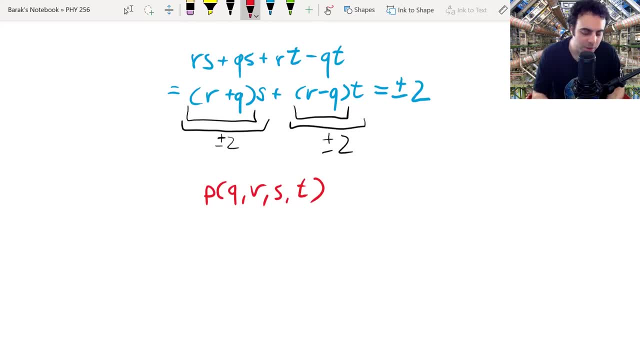 one of these values, So like P of Q equals to plus 1, R equals to minus 1, S equals to plus 1, T equals to plus 1 equals to some number, which is the probability to measure all of those values. So I mean we could assign: 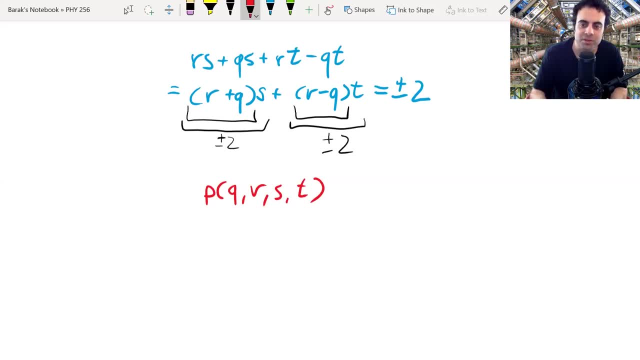 a specific probability, like we could assign, for example, that all the probabilities are equal, So there's a uniform probability of 1 over 16 because there's 16 options. but actually we don't need to do that. The probability amplitude can be arbitrary. we would need the probability to calculate the 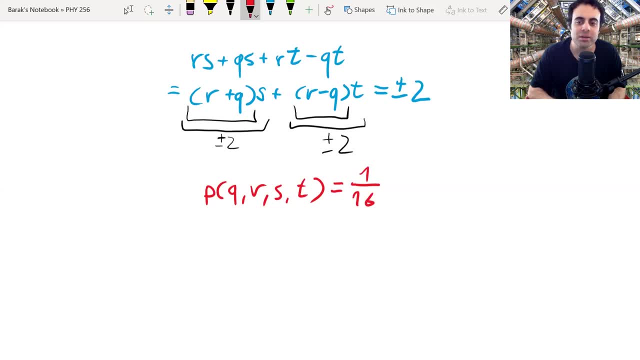 expectation value. but we don't need it if we just want to calculate an upper bound to the expectation value. The externality of the expression number is just the difference between the four properties with respect to the Double nugget Angeles frequency of the vector. 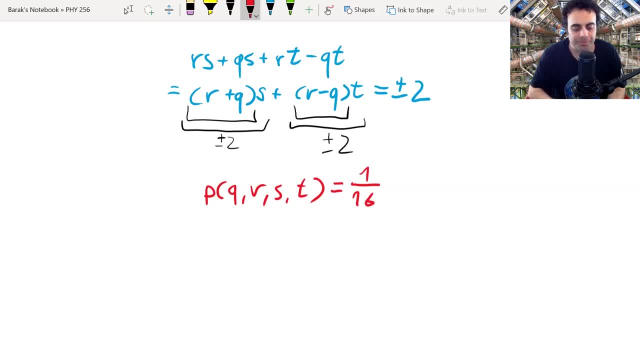 of the interpretation number is just because this variable is usually lower than a P of Q, X, Y, which is equal to a S. P teams are more beyond initial law and big expectation value, which is what we're going to do now. So I have the 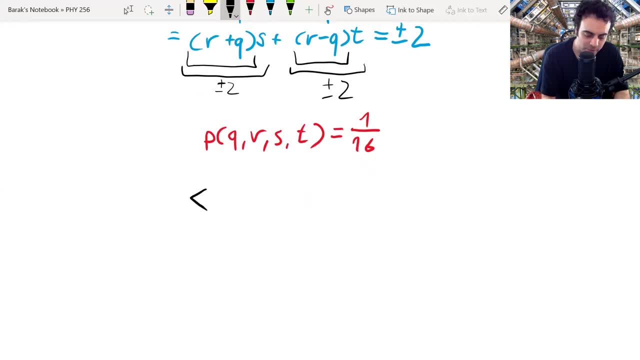 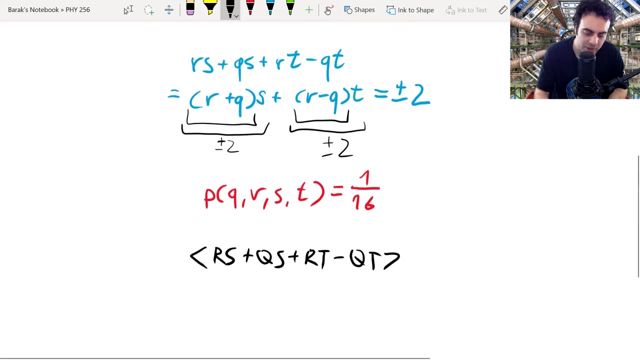 expectation value of this expression that I wrote before, but this time in terms of the actual observables. So this is an expectation value of a particular combination of random variables which we have seen here, yields those values in lowercase and is always equal to plus or minus 2.. So this expectation value is: 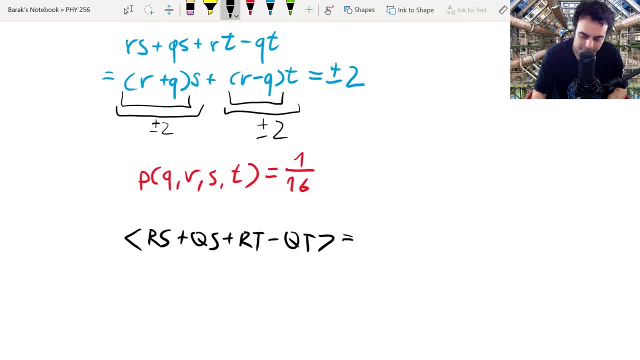 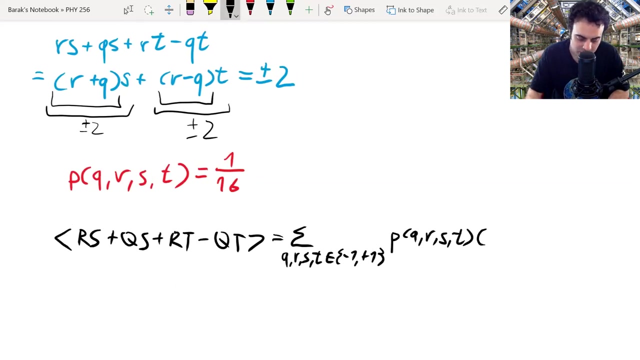 going to be the sum over all the options, q, r, s and t, either minus 1 or plus 1 or мин2.. So the sum is going to be over the probabilities P of q, r, s, t. so the probability to measure some particular values times this combination that I'm. 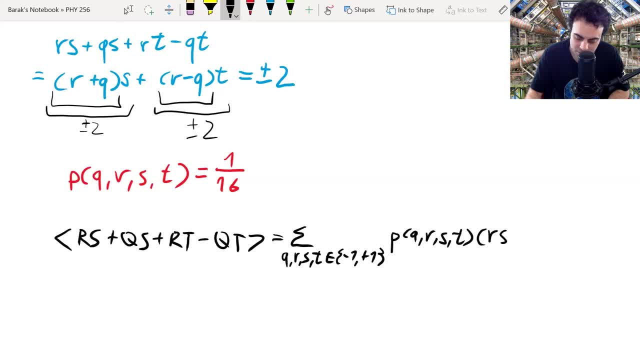 taking into consideration. So I have a question on the chat: what is the difference between the upper case and lowercase letters? So the uppercase and lowercase letters go quickly. I mean there is an indication in the handler mode of USA yhtebra of the, would appear, incidents in this case. 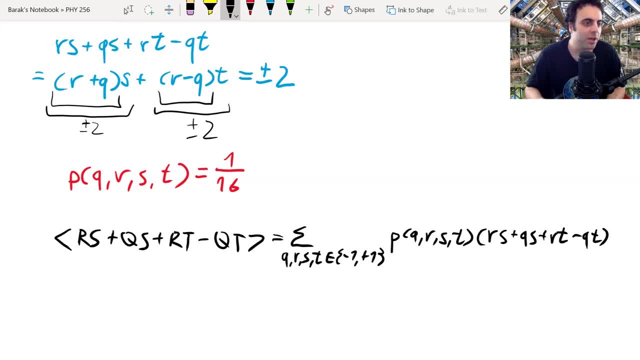 So the upper case has all the buts that mean that there is only one partial value. case letters are random variables. i think it was the second lecture that we learned about random variables. so these are variables that stand for a certain measurement and the result of the measurement is a certain number, plus or minus one. 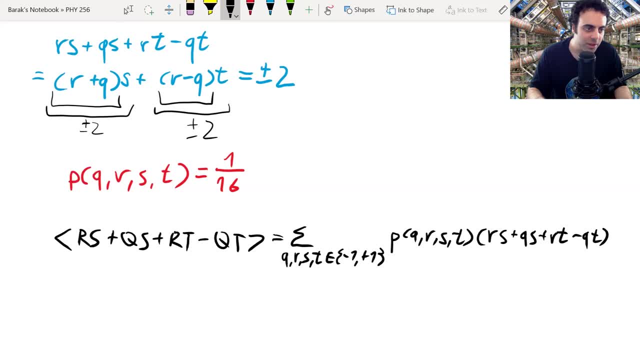 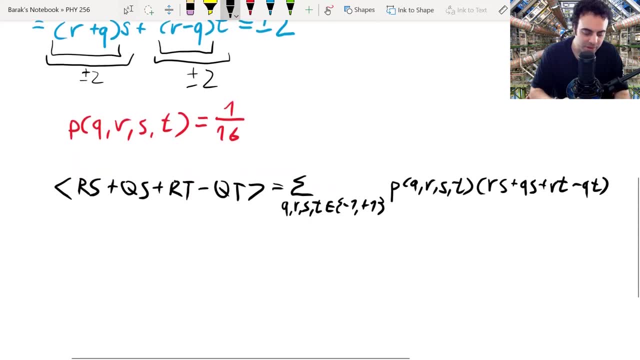 and the lower case is the actual measured value. so remember from the second lecture that we talked about the expectation value of a random variable. uppercase x is the sum over all of the possible values of big x, which we call small x, and then it's going to be the probability for big X to be equal to. 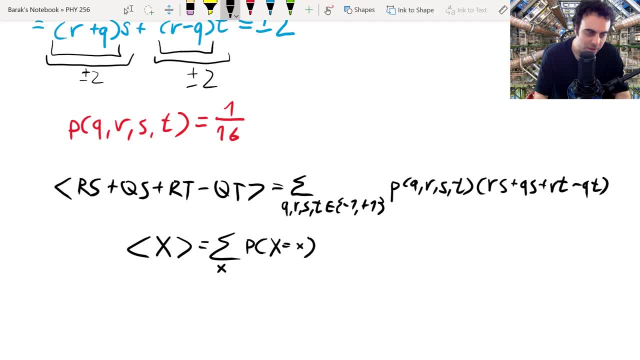 small x, so for the random variable to be equal to the actual number small x times the value X. okay, so this is exactly what's happening here too. this is an expectation value of a certain combination of random variables, and to calculate it I need to sum over all the possible combinations of the measured. 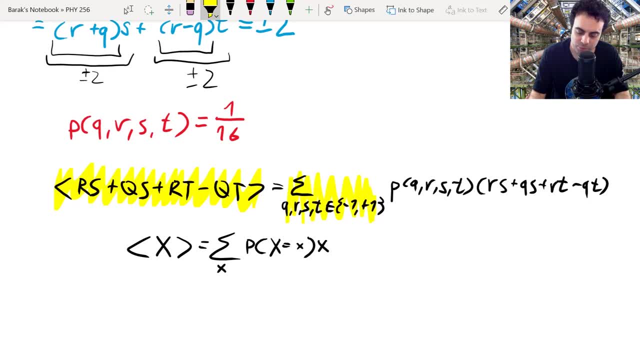 values, which are the lowercase letters, times the probability to measure that value. so this is actually the probability for big Q to be equal to small q, and being out to be equal to small are, and so on, times the actual measure of value which again is encoded in these lower case letters. so now 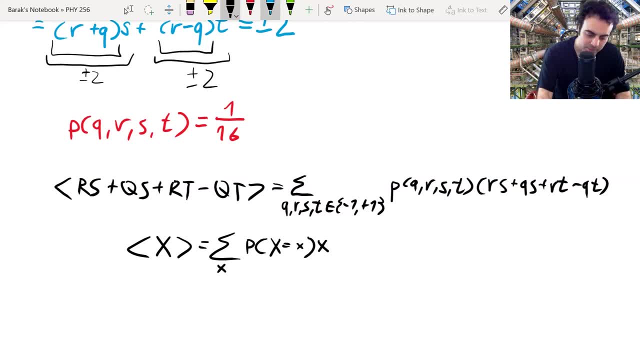 now, since we know that this combination of the measured values is equal to either plus or minus 2, then in particular, we know that it is less than or equal to 2. if it's 2, then it's equal to 2, and if it's minus 2, then it's definitely less than 2. so what we know for sure is that this whole 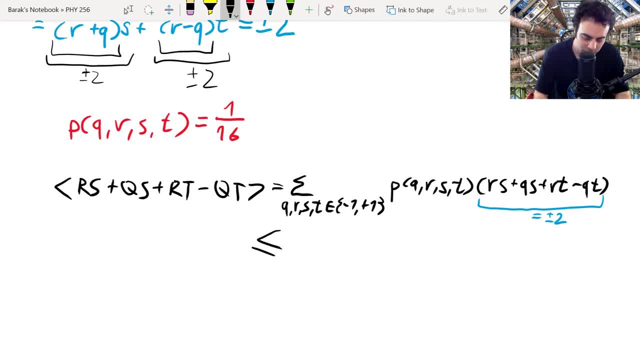 expression is less than or equal to 2 times the sum over q, r, s and t in these particular combinations of plus 1 and minus 1 times the probability to measure these particular values right? so we just said that this is a sum over numbers. each of them is either plus or minus 2. 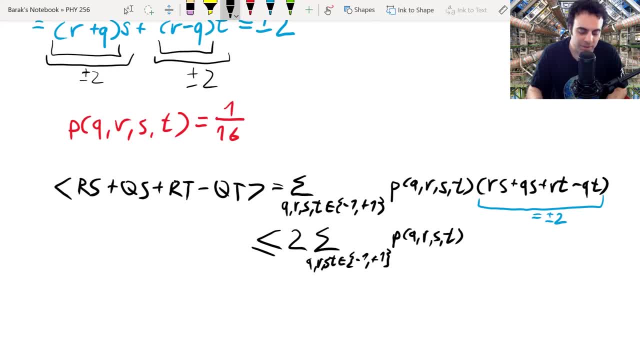 times the probability, then each of them is definitely less than or equal to 2 times the probability. if it's plus 2, then it's just going to be equal to 2 times the probability. if it's minus 2, then it's just going to be less than 2 times the probability. and now, who can tell me? 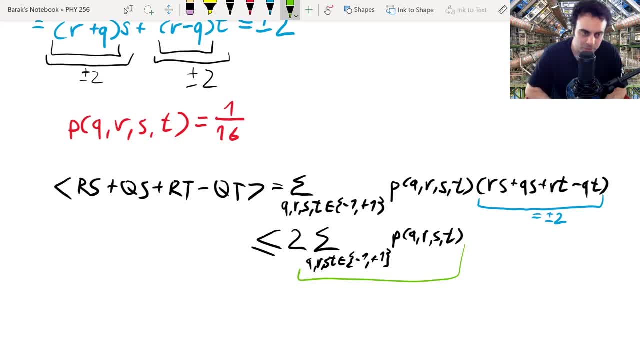 what is this sum? equal to, yes, very good. so it is equal to 1, because the sum of all the probabilities of course has to be 1, which means that this whole thing is just less than or equal to 2. so now we can also use the fact that the expectation value is less than or equal to 2. 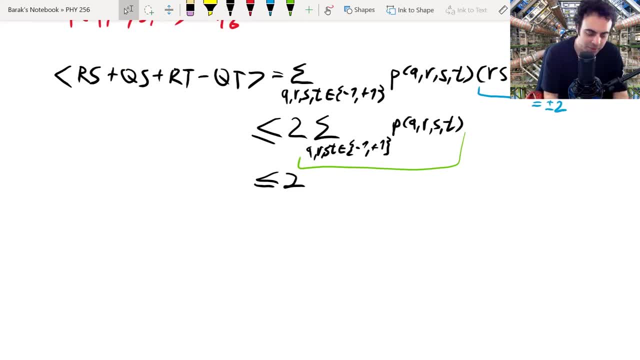 it is linear, so we can actually separate it into different expectation values. so r s plus q s plus r t minus q t is going to be less than or equal to 2. this equation inside the box is called inequality, or sometimes the CHSH inequality. so more generally there's 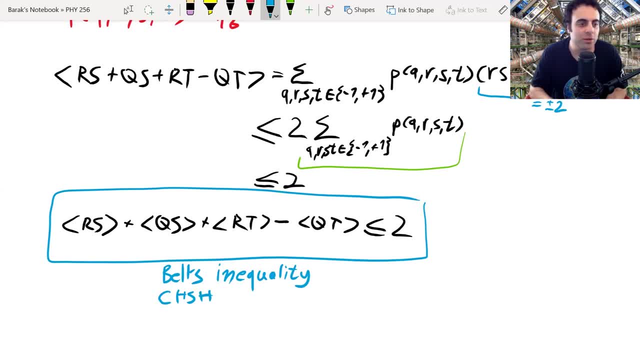 lots of different Bell's inequalities that you can prove for different kinds of observables, and this particular one is called the CHSH inequality, but it is a type of Bell's inequality. so, to summarize, we proved that in any locally realistic theory, the expectation value that we considered here must be less. 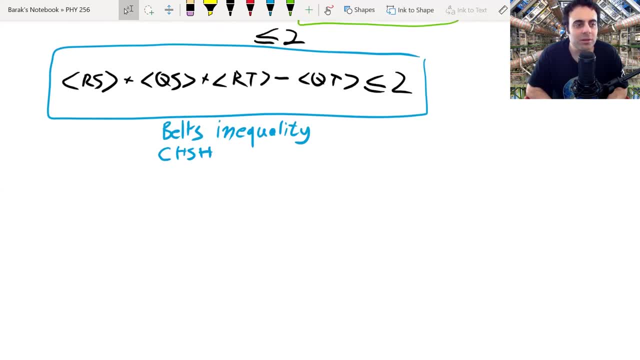 than or equal to 2? there's a question on the chat. so this equation works for general physics, right? I wouldn't say general physics. it's a general physics, but in general it's not a general physics, but it's a. It works for a locally realistic theory. so it works for a classical theory and more. 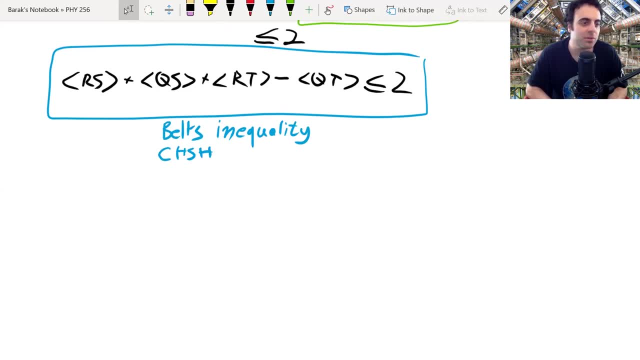 specifically a classical relativistic theory, because it has to be local, so information cannot travel faster than light, which in Newtonian mechanics for example, is possible, Like in Newtonian gravity. if the sun disappears, then we immediately sense a difference in 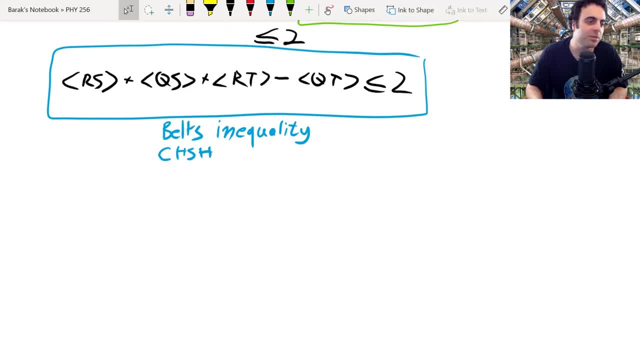 the gravitational field, while in relativity, if the sun disappears, that information actually takes, I think, 8 minutes to get to us, because we are 8 light minutes away from the sun. So this works, this inequality works for classical relativity and, more generally, for any local 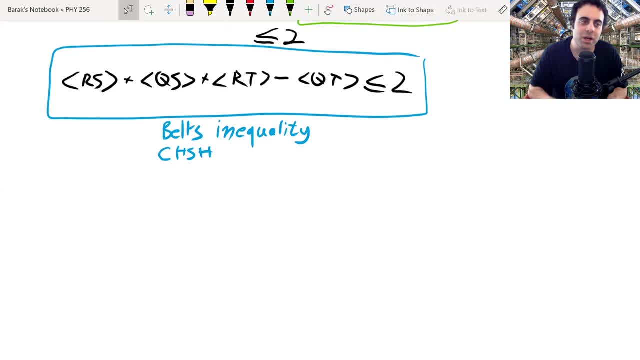 hidden variable theory. But we'll now show that it doesn't work for quantum mechanics. So let's see what happens in quantum mechanics. So let's say I prepared the two qubits in the Bell state beta11,, which says that if the first qubit is 0, then the second qubit has to be 1.. 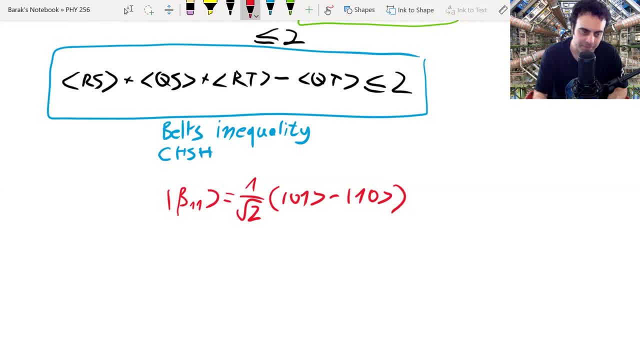 If the first qubit is 1,, then the second qubit has to be 0. Now Alice gets the first qubit and Bob gets the second qubit, And we define these four observables, qrs and t, in terms of the Pauli matrices. 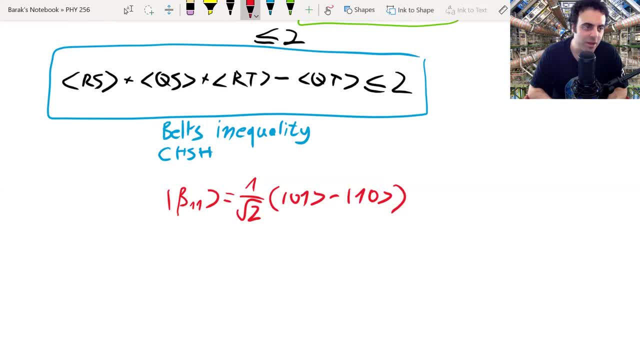 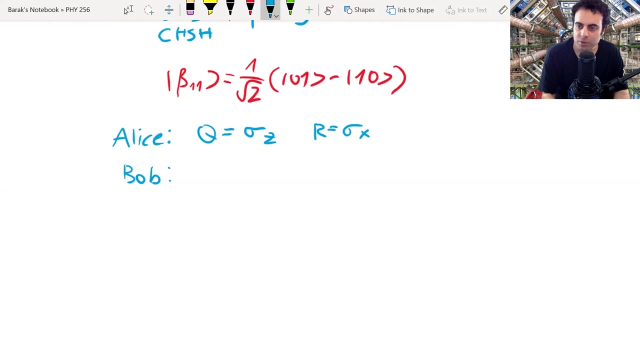 So Alice will take q to be sigma z And r to be sigma x, and Bob will take a bit more complicated combination. And Bob will take a bit more complicated combination, So he will take moras' quasimeter, QU becomes sigma x. 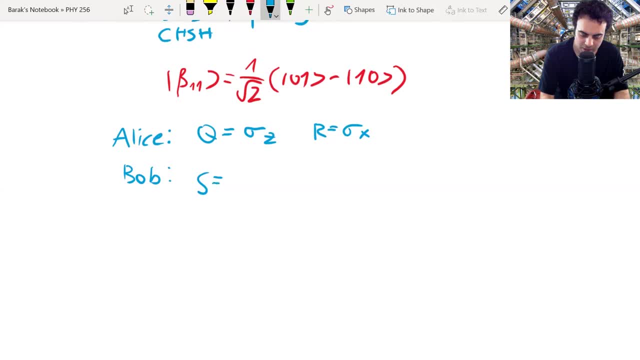 So Q'ds to be is sigma x And R's squalene will take s, equal to minus 1 over square root of 2 sigma x plus sigma z, and t equal to minus 1 over square root of 2 sigma x minus sigma z. Now you will prove, I think, either in the tutorial or the. 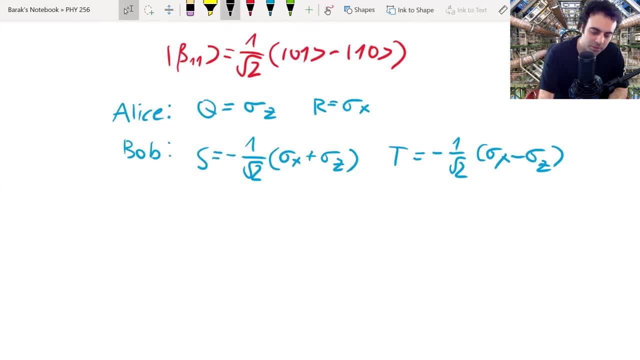 homework that when calculating the expectation values using the rules that we learned about expectation values in quantum mechanics, you get that rs and qs and RT are all equal to 1 over square root of 2 and qt is equal to minus 1 over square root of 2.. So if I take this and I plug it into this formula, 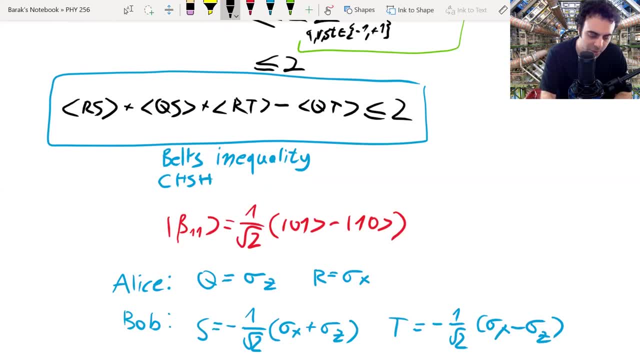 then the first three are going to be equal to minus 1 over square root of 2.. going to be 1 over square root of 2. and last one is minus 1 over square root of 2, but there's a minus sign in front of it, so it's actually 4 times 1 over square root of 2. so in other words, 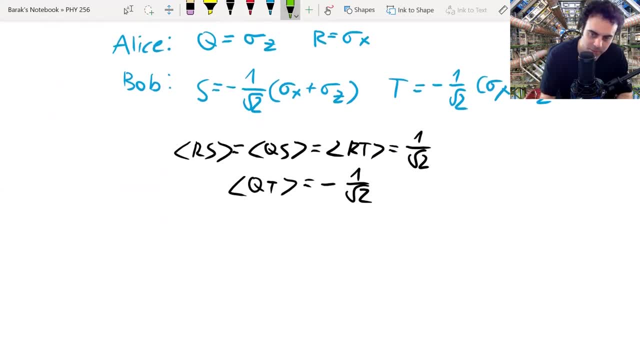 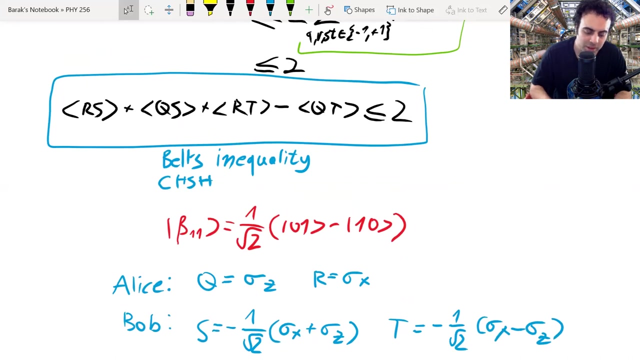 we get that rs plus qs plus rt minus qt is equal to 2 square root of 2, which is approximately 2.8. so so so this is definitely larger than 2, but we've proven here that with the assumptions of local realism, the combination has to be less than 2. 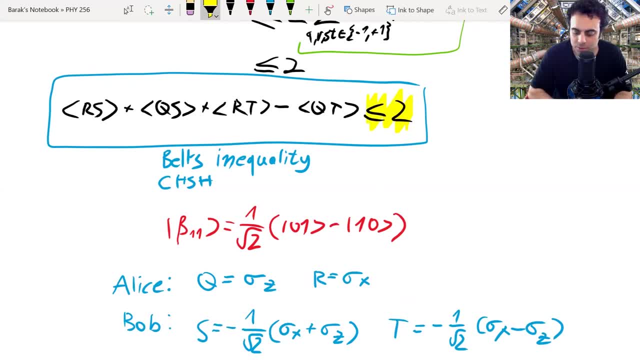 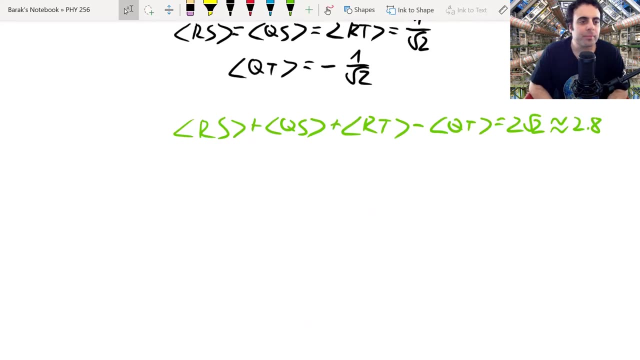 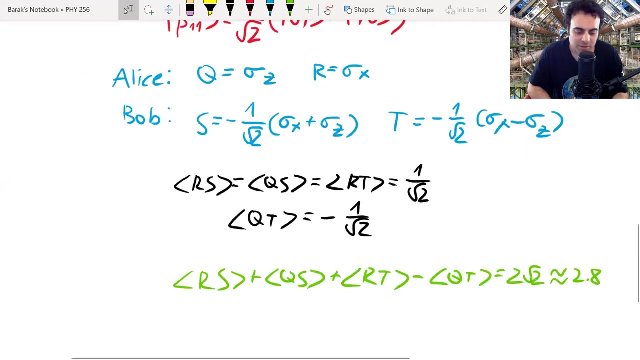 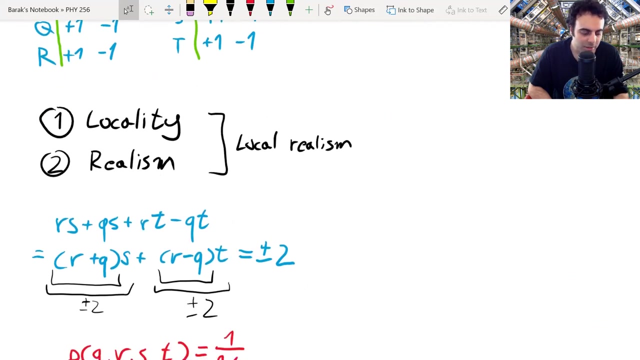 in other words, quantum mechanics, violates bell's inequality and therefore the assumptions of locality and realism. at least one of them has to be incorrect. so i have a question on the chat. why was that concluded from that answer? so i had two assumptions, locality and realism, and these assumptions allowed me to calculate the expectation value. 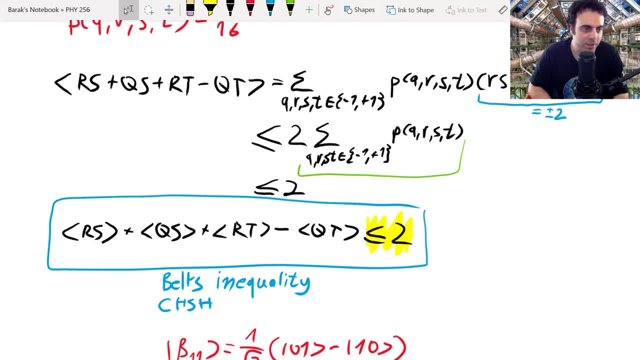 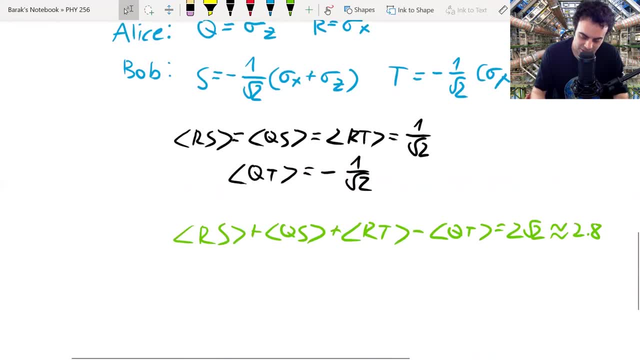 classically and i got that the expectation value has to be less than or equal to 2, but now we see that in quantum mechanics the expectation value is actually larger than 2, which violates bell's inequality. therefore, these two assumptions- at least one of them has to be. 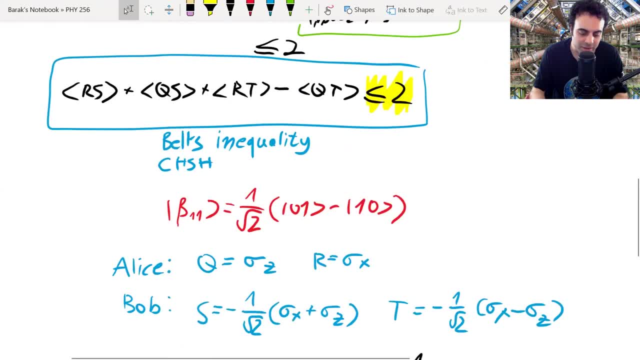 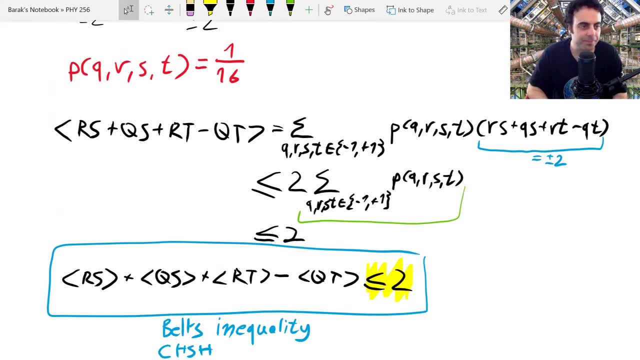 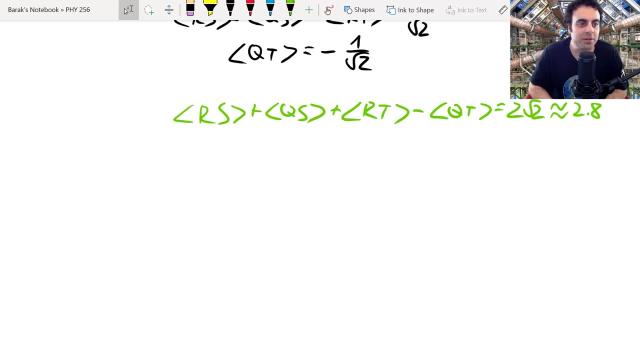 incorrect to explain why this calculation we did here is actually not applicable to reality. so, importantly, this is a very important question. because it's a very important question, because it's not just a theoretical result. there have been many different experiments over the years and they have verified that bell's inequality is actually violated in nature. so this means again that our 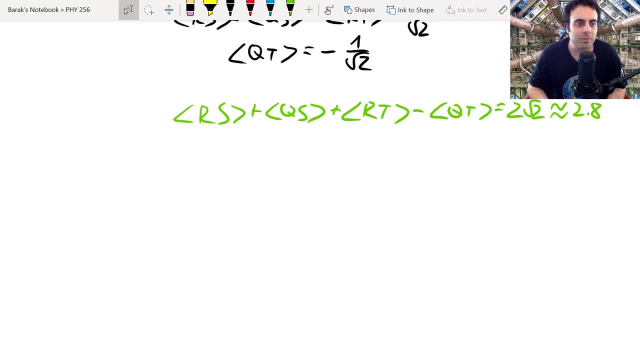 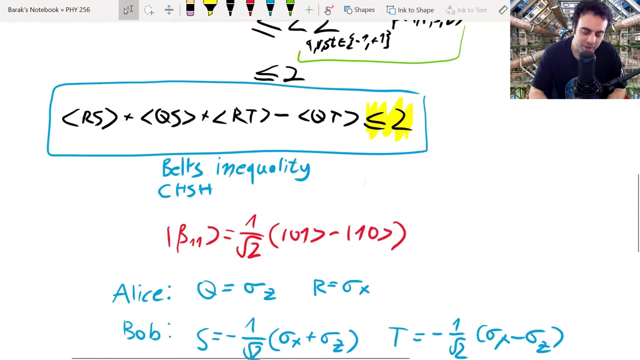 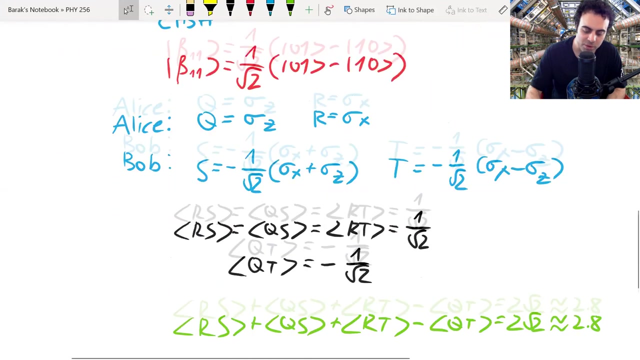 assumptions- either locality or realism, or both, must be incorrect. it also means that quantum entanglement is stronger than classical correlation, which is locally realistic, because with classical correlation the best you can do with this expectation value is two. two is the largest value you can get. but quantum mechanics is somehow stronger in that it lets you actually go beyond that. 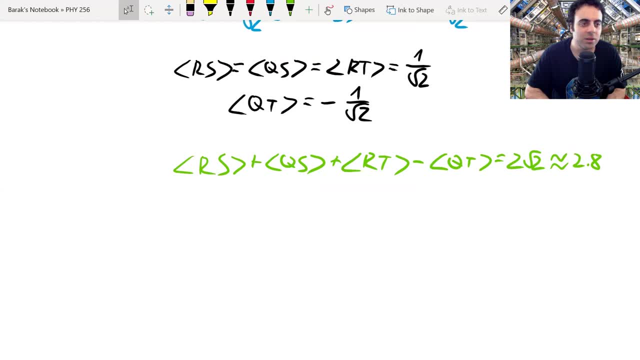 and the maximum value you can get turns out to be 2.8 instead of two. so well, intuitively, this is kind of a numerical way to show that entanglement is stronger than classical correlation. but also, as we will see soon, entanglement allows us to do all. 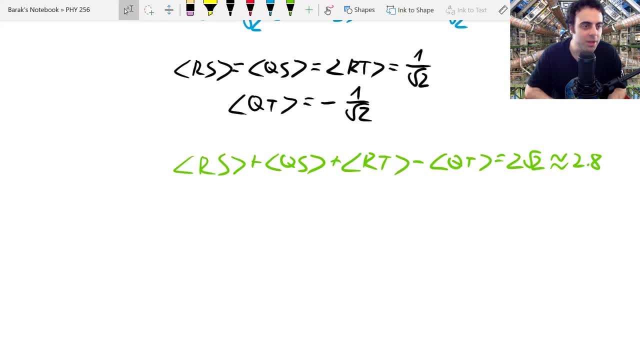 kinds of very interesting and useful things that we can't do with classical correlation. in particular, like i said before, quantum entanglement is what makes quantum computers work potentially faster than classical computers, because in classical computers the bits can be correlated classically, but in quantum computers 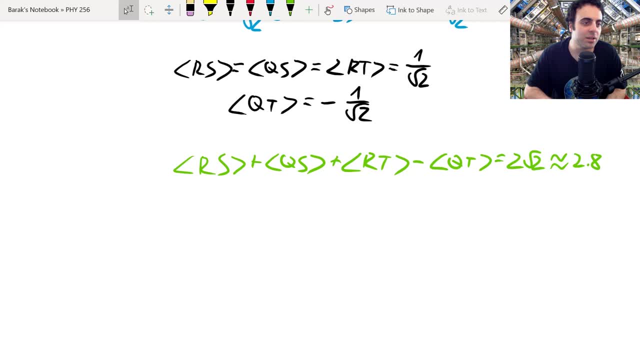 the bits are now qubits and they can be entangled, so this pretty much rules out any local hidden variable theory and instead we have two options: either locality is an incorrect assumption, but realism is correct in this case, we get a non-local hidden variable theory where the non-local means 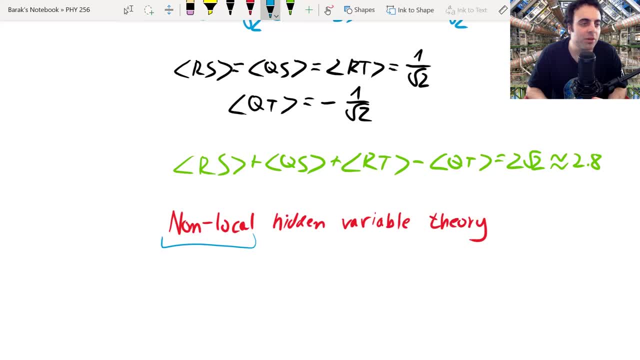 that now we do allow information to be transmitted faster than light or even instantaneously, and the hidden variable part means that this is still a deterministic theory, so it satisfies the assumption of realism. so one example of a non-local hidden variable theory is a theory that i mentioned in the past and it's called the broy-bomb theory. 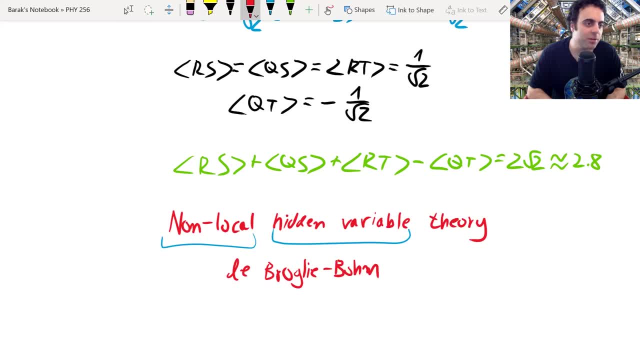 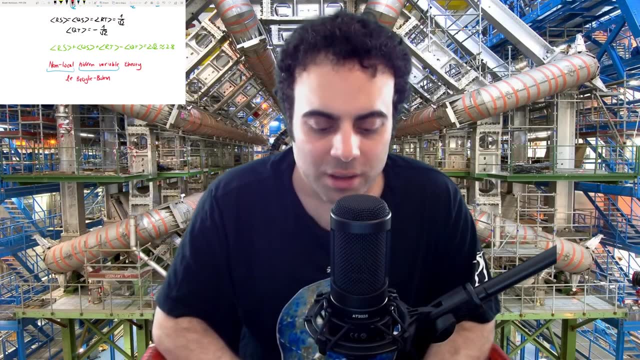 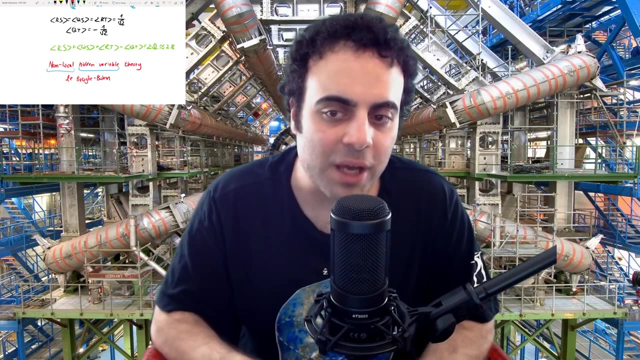 and now this is just one example, but it is the most common example that people usually consider for non-local, hidden variable theories. now, in this theory, the state of each particle depends on the states of every other particle in the universe, so somehow every particle needs to know what's happening with every other particle in the 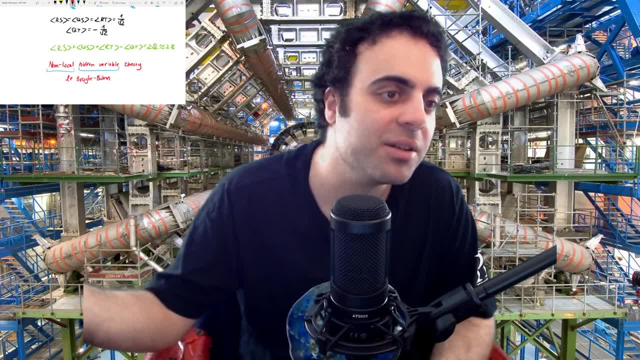 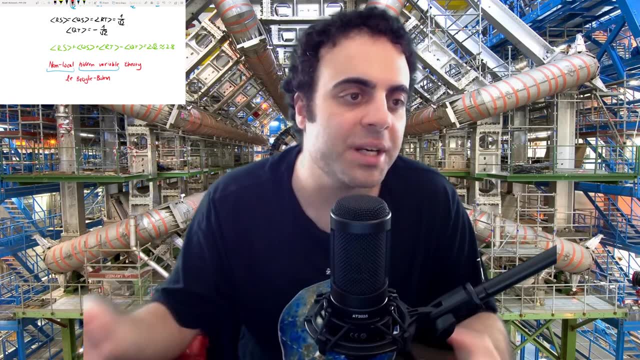 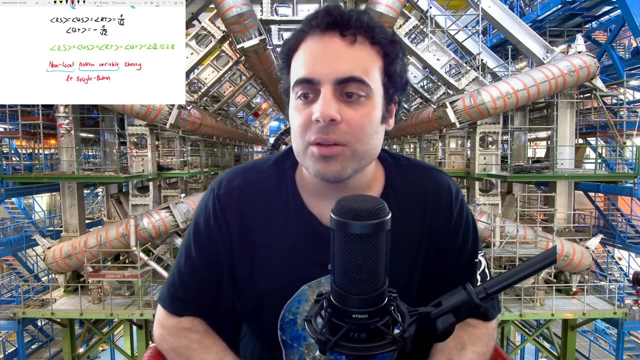 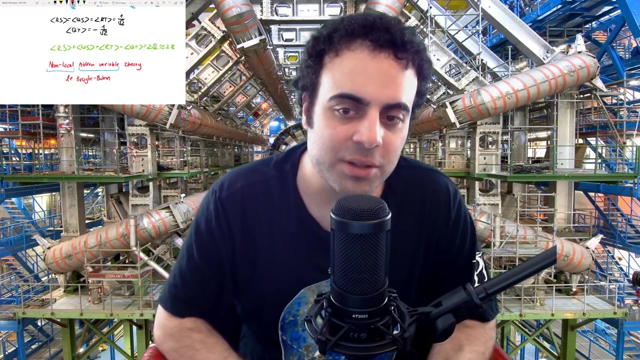 universe, even if it is in the andromeda galaxy or even if it's actually outside of the observable universe, in a place where we can never actually reach unless we can travel faster than light. so most physicists don't like this kind of theory, because those theories tend to be complicated. 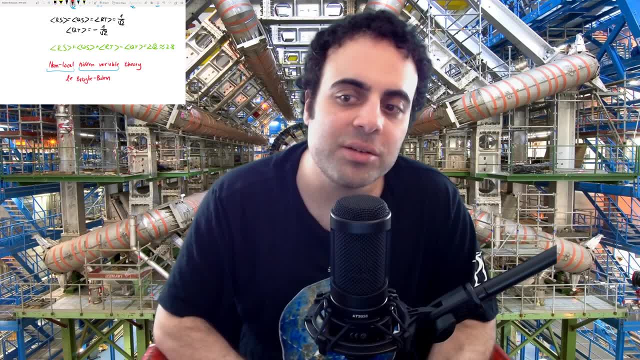 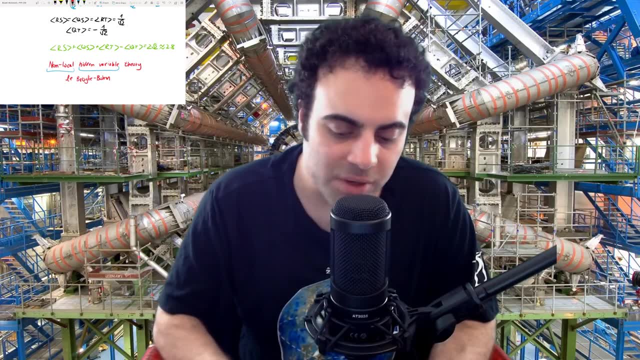 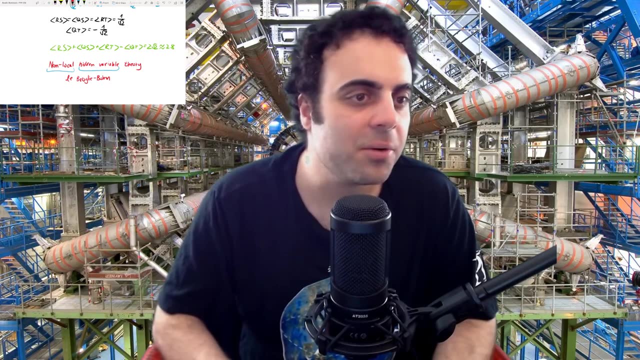 and contrived and they lack the simplicity and elegance and universality of quantum theory. so quantum theory is very simple: it's just vectors in a hilbert space and that's basically the whole theory. but those are not quantum theories. The Breuil-Bohm theory: I'm not going to teach you about it, but you can look it up on Wikipedia, for example. 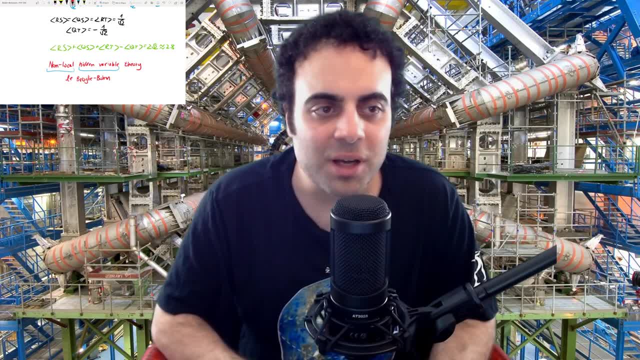 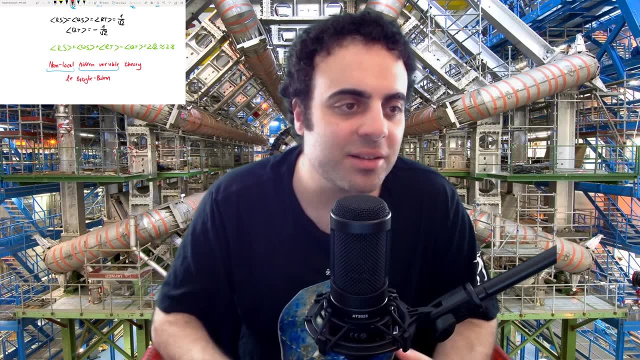 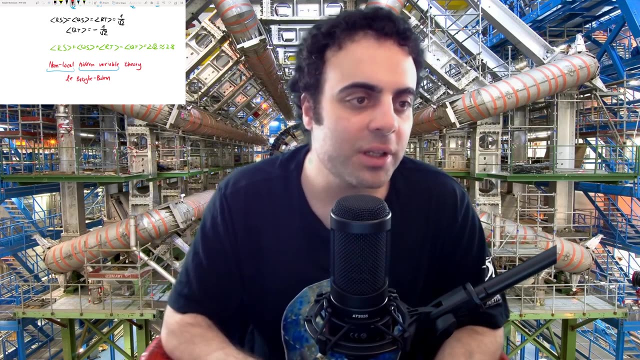 and you can see that it has kind of- I would say- ugly equations that don't really have this elegance and simplicity of quantum mechanics. Also, if we do have a non-local hidden variable theory, and this means that this would be the spooky action at a distance that you hear about all the time- 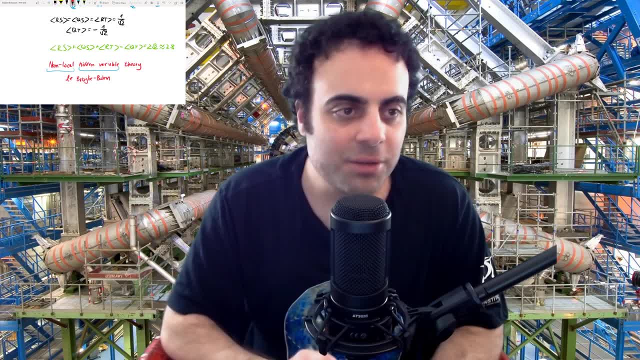 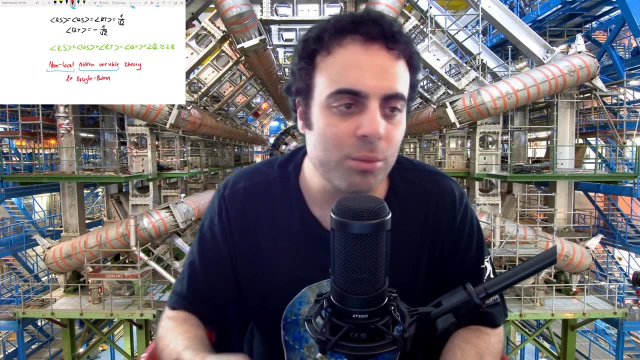 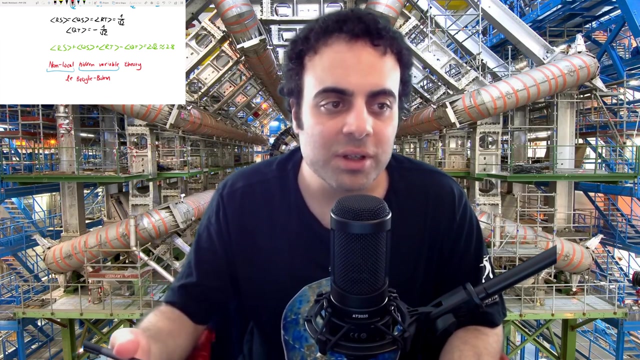 but notice that even if locality is violated, it still doesn't necessarily mean that faster-than-light communication between people is possible. So communication between two people requires a form of non-locality that is controllable. It requires Bob to be able to choose which state he measures and by doing that send a message to Alice. 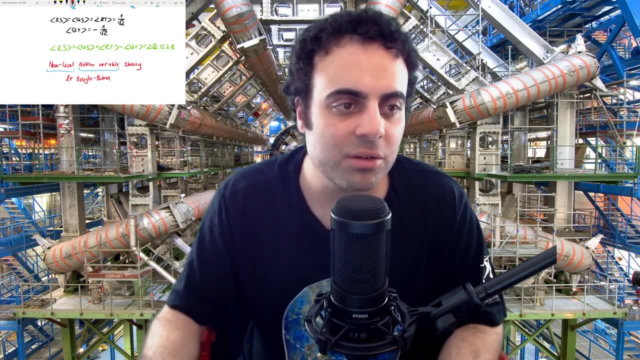 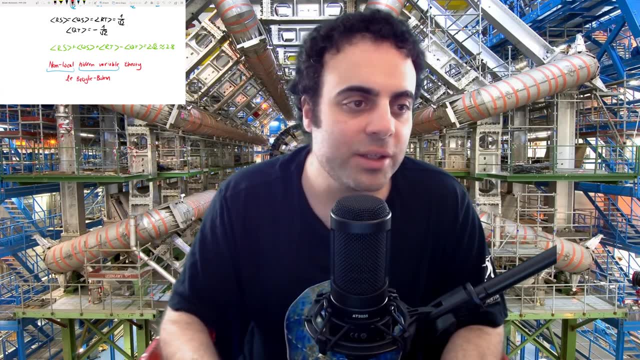 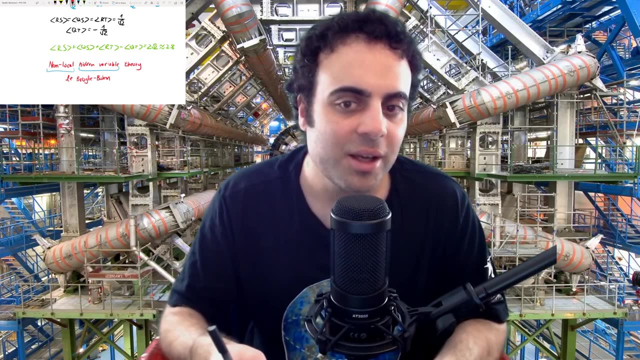 And then when she measures her qubit she will discover the message. So a theory can be non-local but still not allow any communication faster-than-light. So somehow the qubits themselves would know about each other's states. but it doesn't mean that Bob can actually control what he measures. 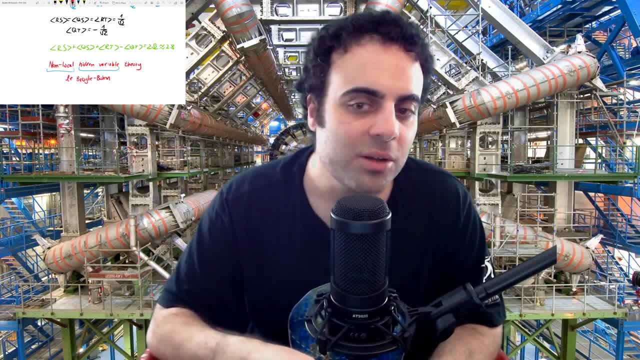 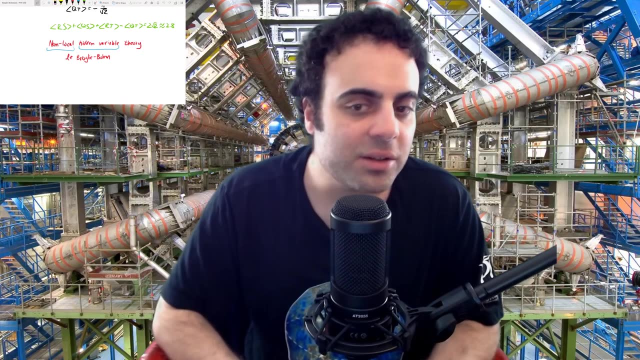 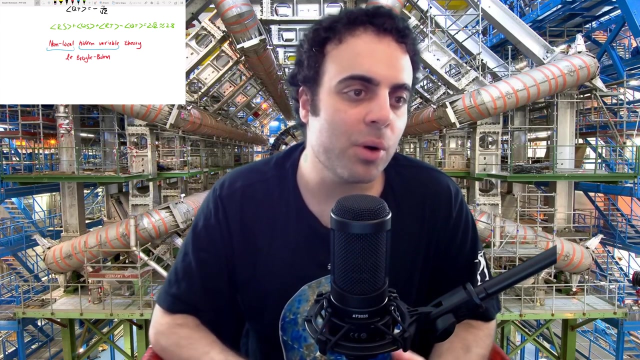 so that he can send a specific message to Alice. So this doesn't violate the no-communication theorem that we discussed, and it also doesn't violate relativity. Now the second option is that realism is the incorrect answer. This is a very common assumption, but locality is correct, or maybe even that both are incorrect. 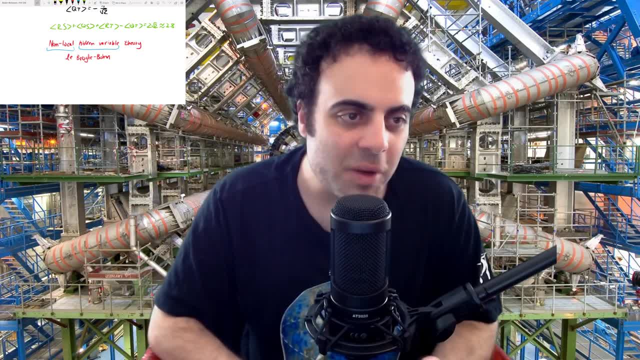 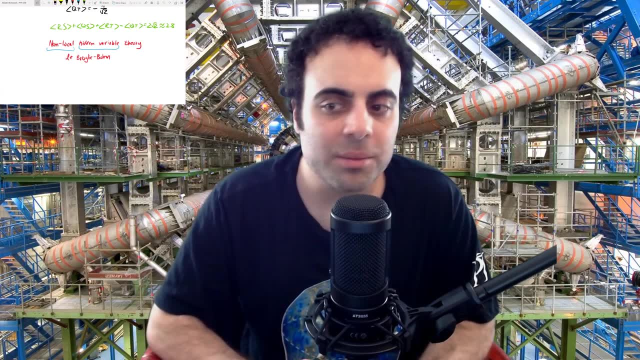 And this is the option that most physicists prefer, even though it's less intuitive and it contradicts our experience with the classical world. So definitely, if you open the fridge to get an apple, the apple has always been there. Even before you open the fridge to get an apple, the apple has always been there. 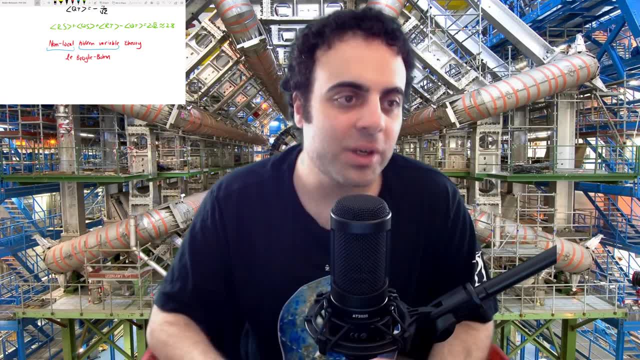 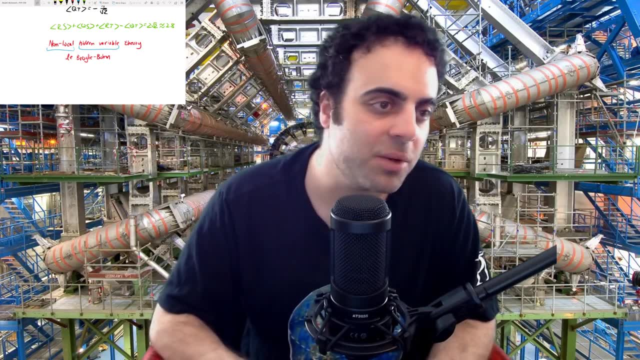 Even before. you observed it right. This is how classical physics works. It is deterministic. There's no way that you open the fridge and there's like a 50% chance to get an apple and a 50% chance to get an orange. 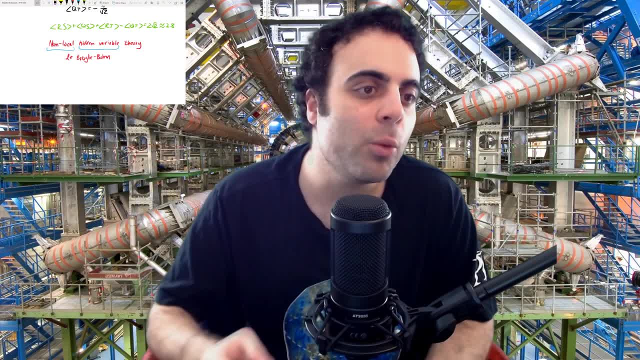 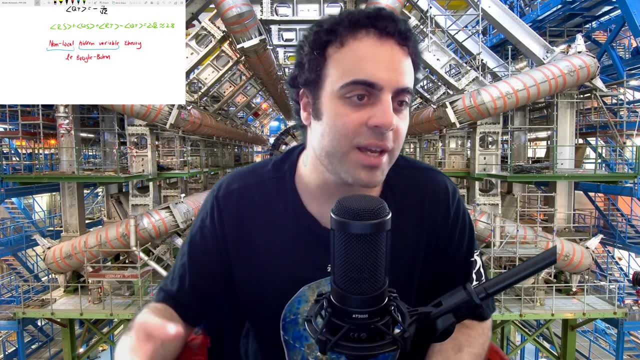 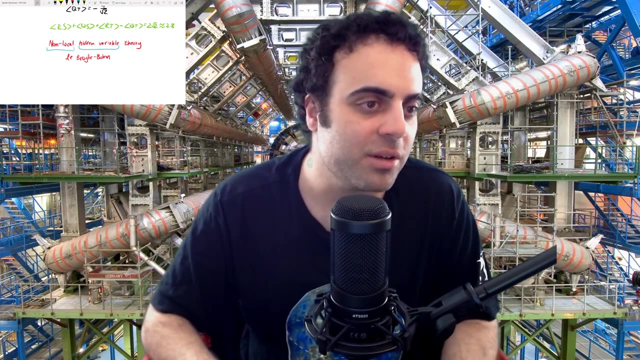 There's always gonna be an apple, and that apple has always been inside the fridge even before you opened the fridge. It was just a hidden variable until you opened the fridge and measured what kind of fruit is inside the fridge. Okay, But it was always an apple. 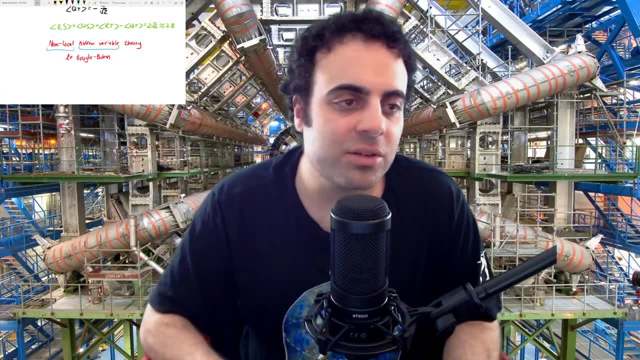 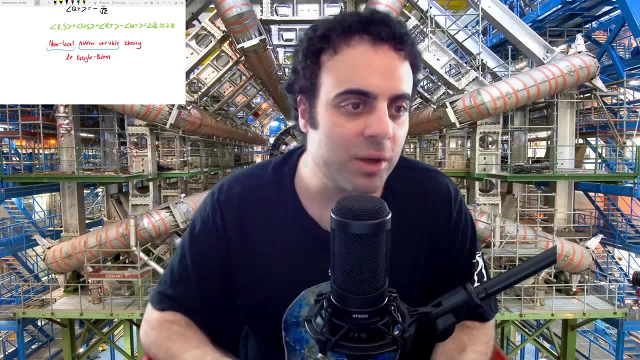 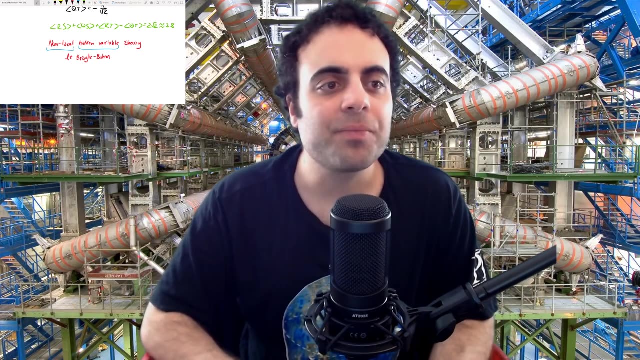 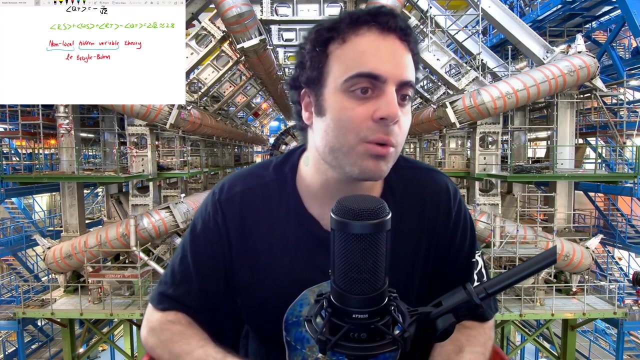 But the same it, just it doesn't have to be true for a qubit. Most physicists agree that the way that quantum mechanics works means that when you measure the qubit it is a non-deterministic measurement. You have a certain probability to measure zero or one. 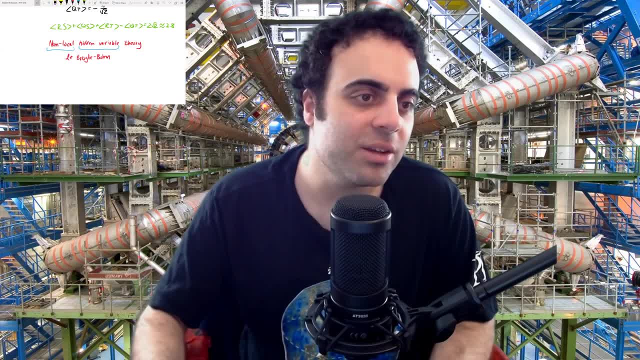 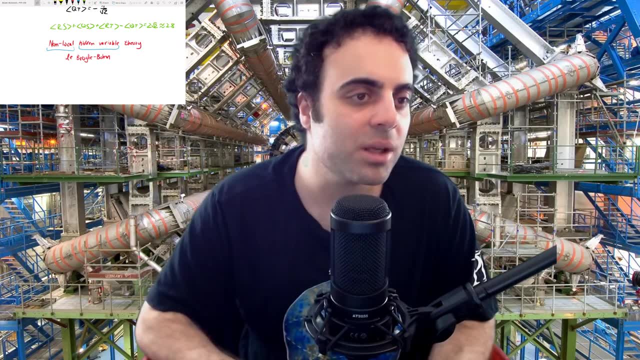 You have a certain probability to measure zero or one. You have a certain probability to measure zero or one When you do the measurement. it was not in any one of those specific states. It was just in a superposition until you made the measurement. 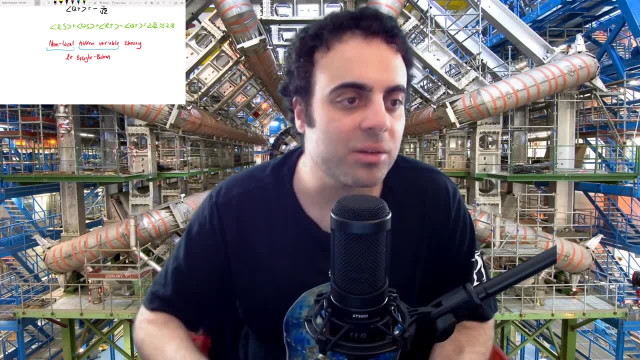 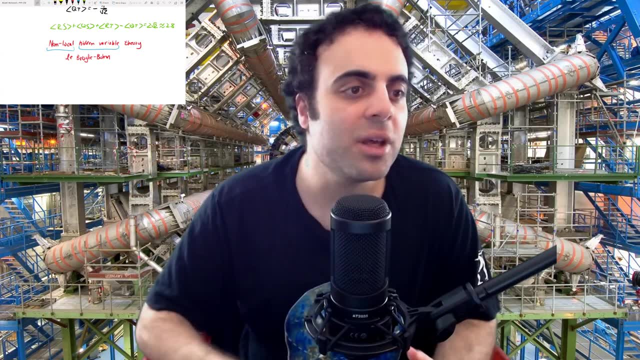 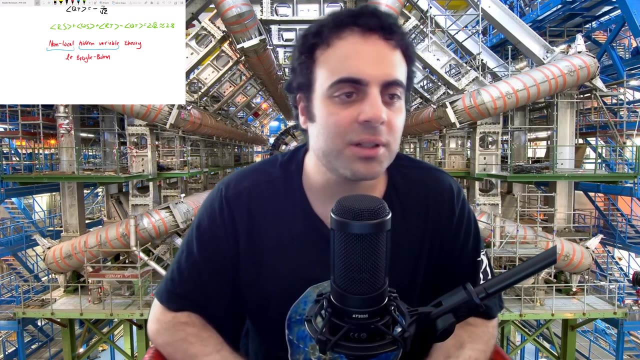 This is what a theory that doesn't satisfy the realism condition is. It's a theory where things are not predetermined before you make the measurement. Now I know this kind of gets very philosophical, But I think if you want to really understand it, 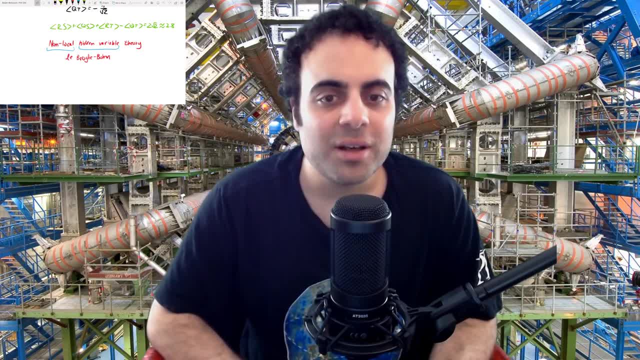 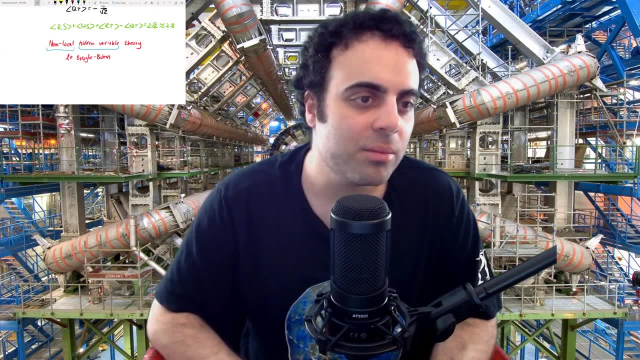 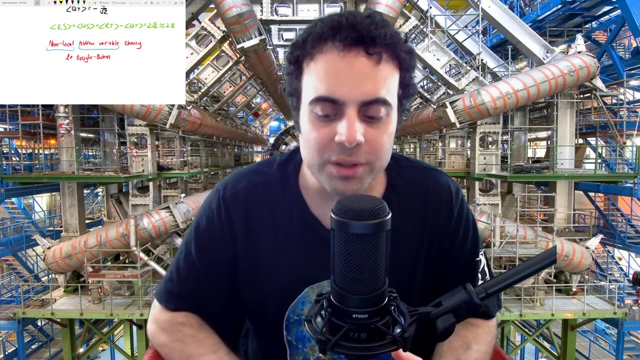 if you want to really understand what quantum mechanics is, then you have to understand this, And usually in a first course on quantum mechanics you don't talk about Bell's theorem, And I think that's a mistake, Because in order to know what quantum mechanics is and how it is different from classical mechanics, 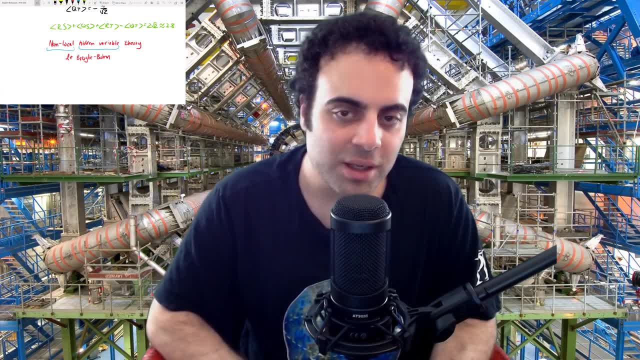 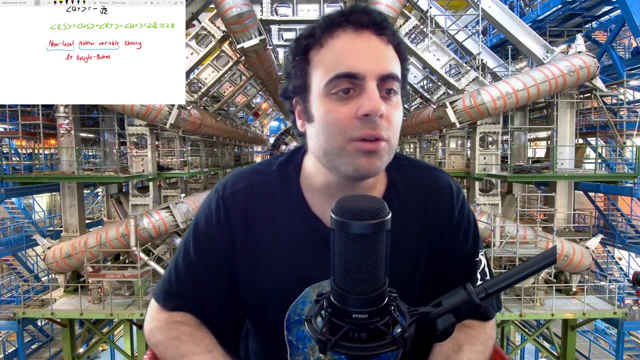 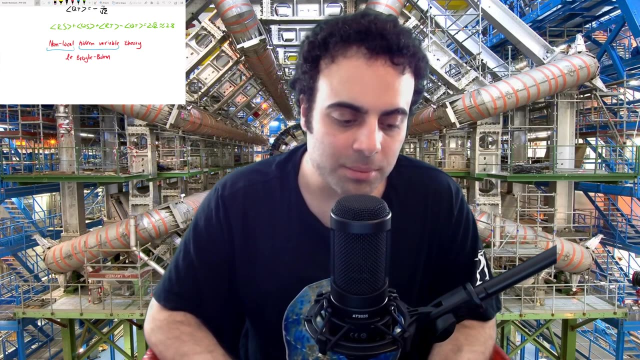 you have to understand that quantum mechanics is a theory that is not deterministic. It doesn't satisfy realism. I have a question on the chat: What about the violation of locality in this theory, Right? so, like I said, what most physicists agree is that realism is the incorrect assumption. 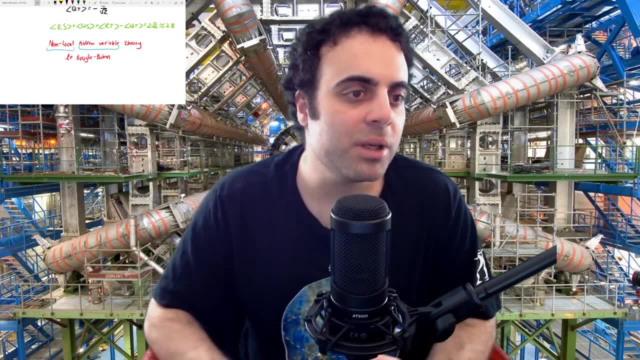 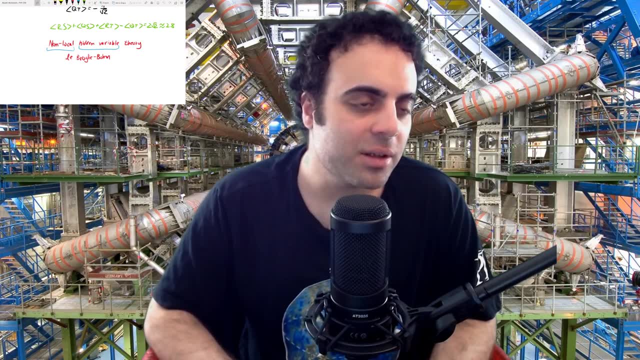 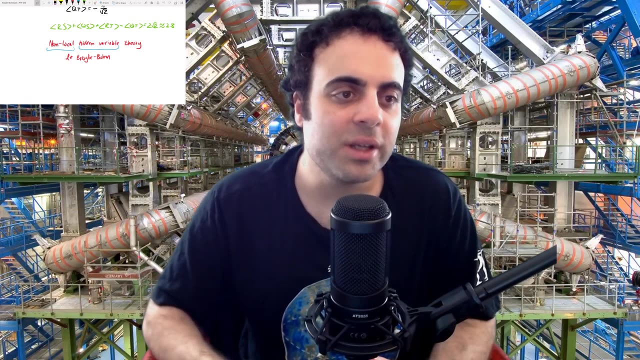 So now, locality may or may not be correct. We are almost 100% certain that you cannot communicate faster than light. So, according to all of known physics, communication faster than light is impossible. The speed of information is limited by the speed of light. So this is a fact that is indisputable. What we are not so sure about is whether you can say that one qubit knows about the state of the other qubit and they somehow communicate between themselves faster than light or even instantaneously. 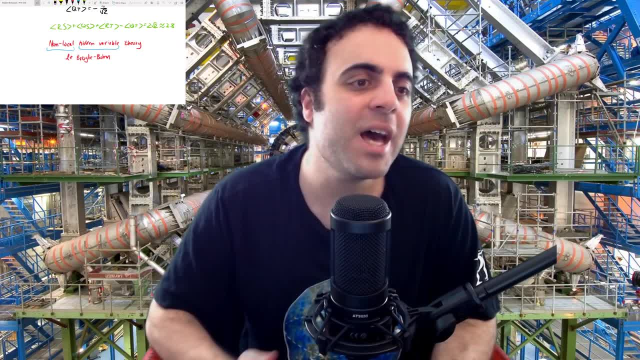 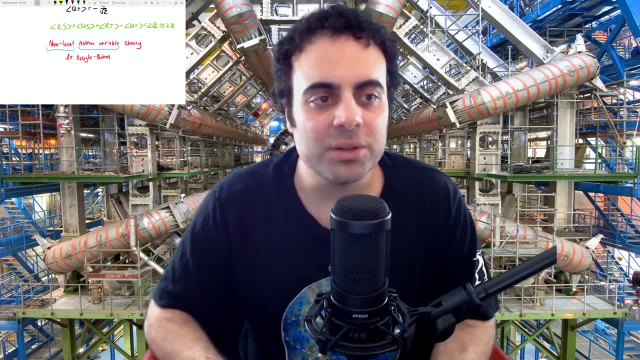 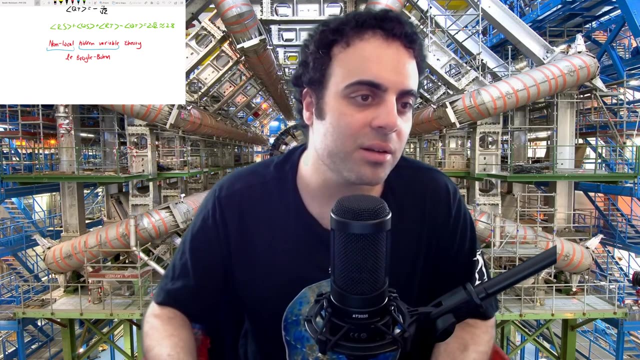 So, like I explained last time, it doesn't actually have to be that way. An entangled state of qubits doesn't depend on the distance between the qubits. It just says that if you measure both qubits, then if one of them is 0, the other is 1.. If one of them is 1, the other is 0. So there's no actual reason to assume that one qubit knows about the state of the other qubit. You can assume non-locality, but depending on how you exactly define locality. 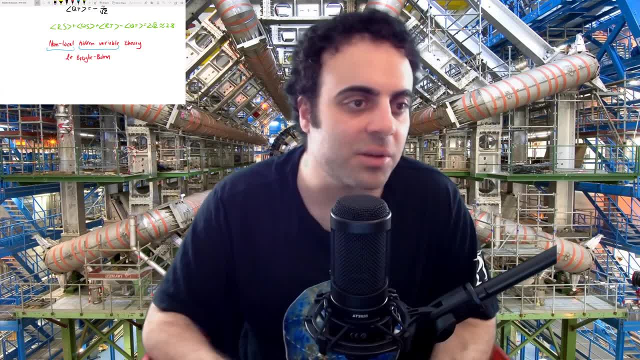 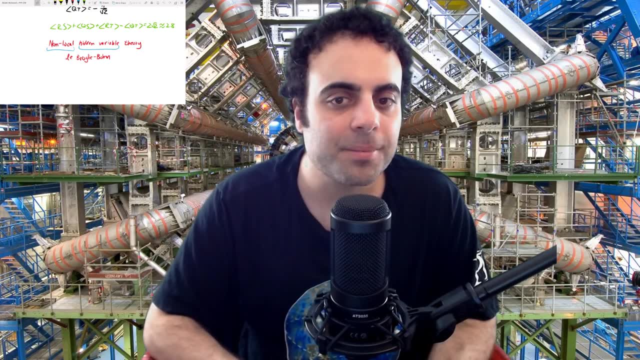 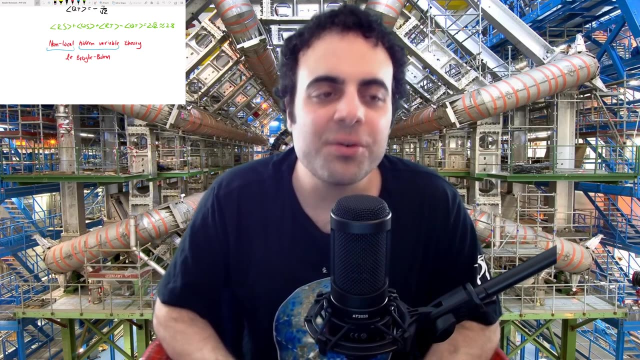 you can say that this either violates or doesn't violate locality, And this is kind of a more complicated philosophical discussion I don't want to get into right now. Another important lesson of Bell's theorem is that there is something fundamentally profound and powerful about quantum entanglement which classical correlation doesn't have. 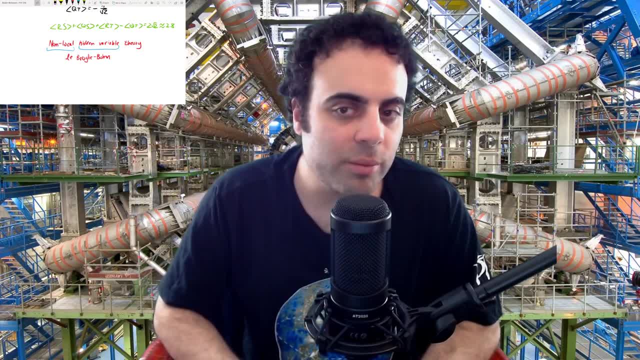 The probability of quantum entanglement is exactly what makes quantum computers more powerful than classical computers, like I said before, And it also has some other interesting applications, like quantum teleportation, which we will discuss later, and quantum cryptography, which I don't think we will discuss here. 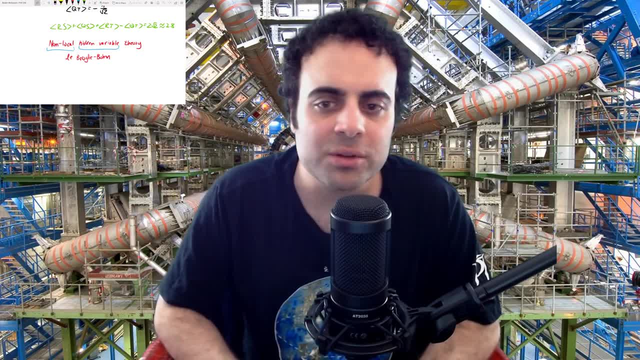 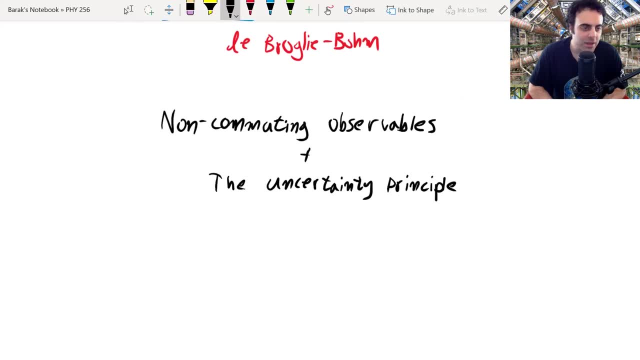 but we may discuss it if we have time at the end of the course. So now I want to talk about quantum cryptography. I want to talk about non-commuting observables and the uncertainty principle. So remember that. well, we haven't defined it in the lectures. 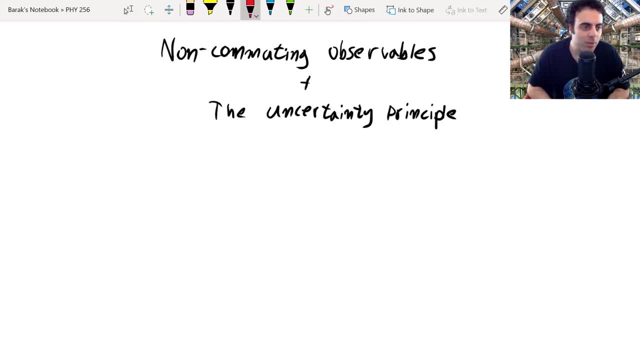 but it is defined in one of the homework problems and I think you talked about it in tutorial as well. There is this thing called the commutator of observables, So it's a commutator of two operators or of two matrices. 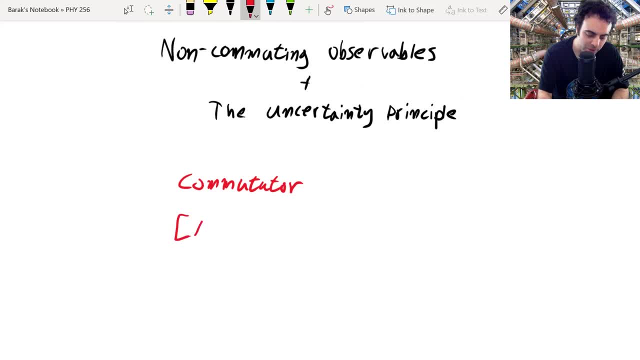 It's defined as follows: So a commutator of A and B is defined as AB minus BA. So if A and B commute, that means that AB equals to BA Operators. commuting means that we can switch the order and still get the same thing. 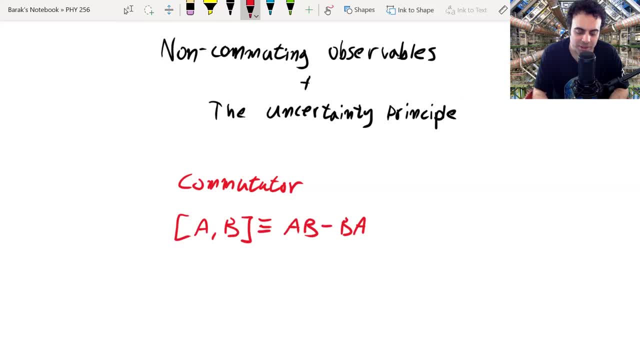 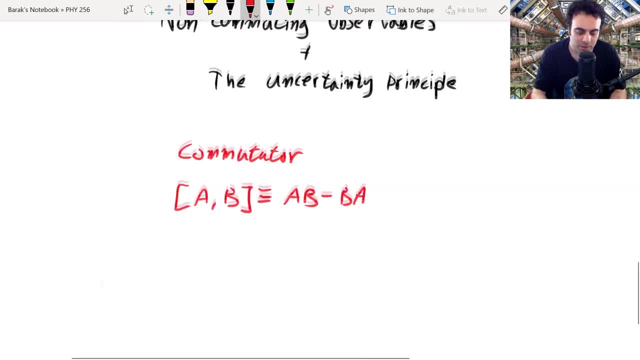 So if they commute, then AB is going to be equal to BA and therefore the commutator is zero. So if AB commutator equals zero, that means that A and B commute, But if they don't commute then AB doesn't equal to BA. 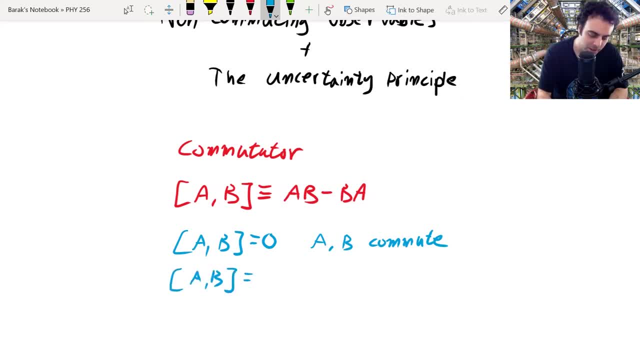 and therefore the commutator of A and B is not going to be equal to zero. Now we will prove all kinds of different properties of commutators in tutorials and homeworks, and you can check the lecture notes to see all of those properties. 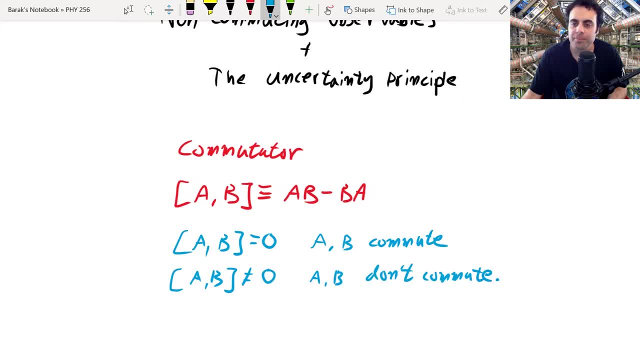 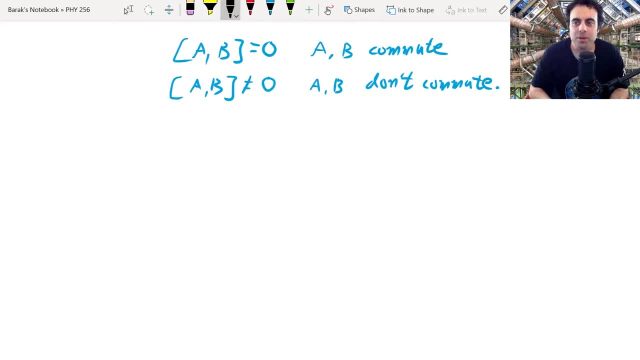 so I won't go into them right now. What I want to talk about now is the uncertainty principle. So when two quantum observables don't commute, we get an uncertainty relation. Now what is uncertainty? Uncertainty is just a fancy name for what we already talked about. 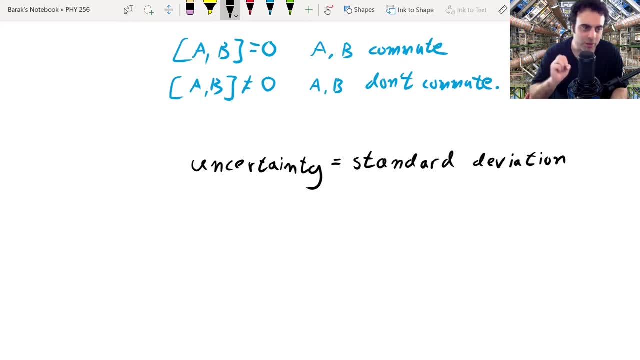 in one of the first lectures, which is standard deviation. So just like a state is actually a vector and an operator is actually a matrix and a linear combination is actually a superposition, then a standard deviation is actually uncertainty, because physicists just like to use 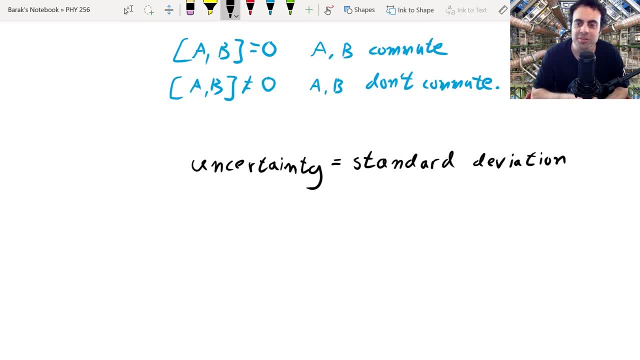 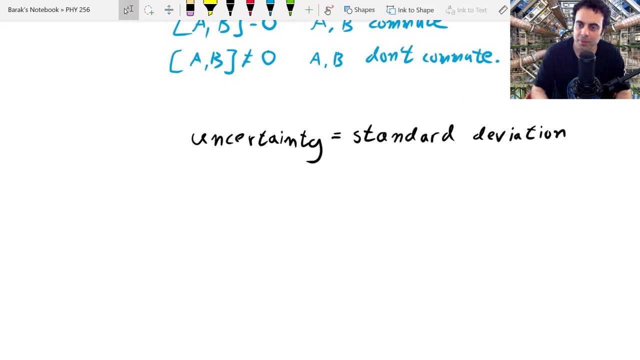 different names for things that already have names, I guess. So the most well-known relation, the most well-known uncertainty relation is the position momentum uncertainty relation that you have definitely seen before, which is that delta x or the standard deviation in position. 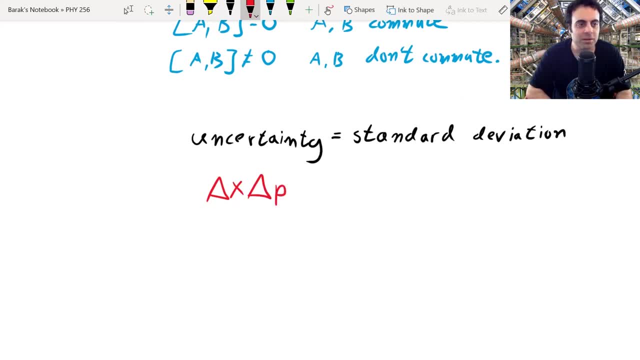 times delta p, or the standard deviation in momentum, is greater than or equal to 1 half. and remember that we are using units where h-bar is equal to 1, so we don't have to worry about writing down h-bar. So x and p are two operators. 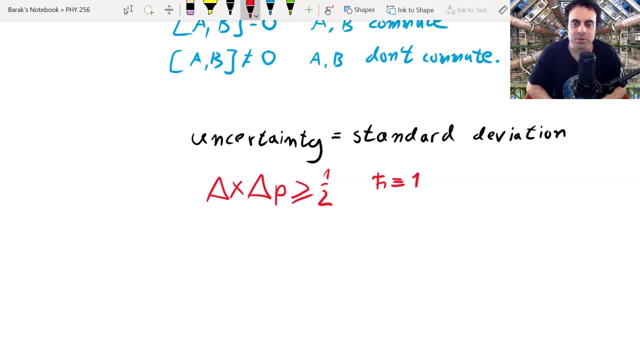 so they are Hermitian operators because they correspond to observables. The observables are position and momentum, and the inequality means that the product, so the product of the uncertainty in position with the uncertainty in momentum, cannot go below 1 half. 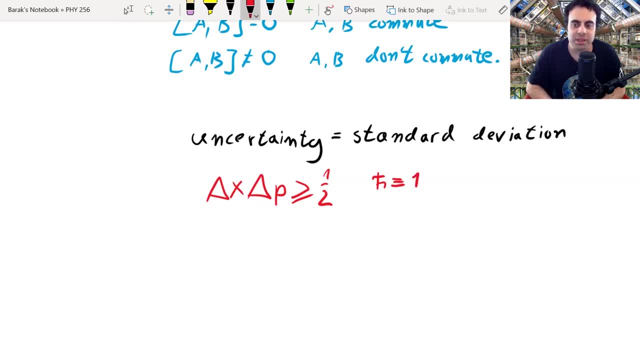 This means that delta x and delta p, they can't both be 0 at the same time. We can never know both the position and momentum with arbitrarily high certainty. So let's prove this relation for the general case of any two observables represented by two Hermitian operators. 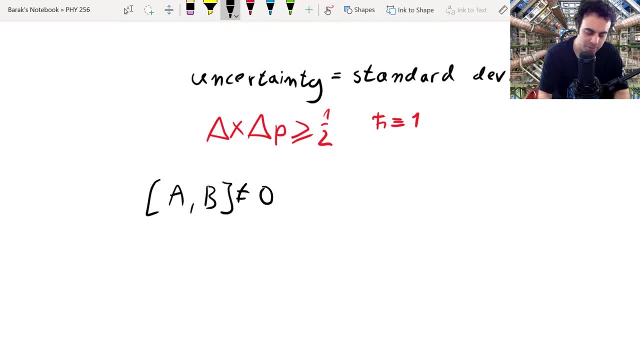 a and b that don't commute. Actually, we can prove it for any two operators, a and b, even if they do commute. but you'll see that if they do commute, then there is no inequality. There is no inequality to talk about. 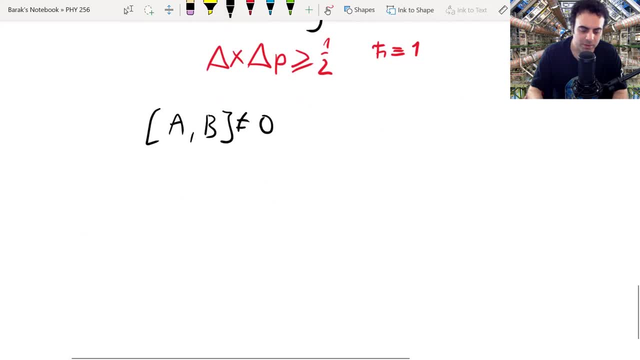 So, first of all, recall, the definition of the standard deviation is that delta a, the standard deviation in a is the square root of the expectation value of a minus expectation value of a squared. Okay, Let's take the square of this. 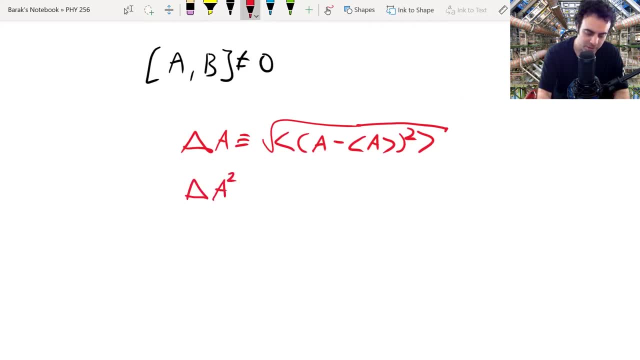 So delta a squared is expectation value, a minus expectation value a squared. Now, in quantum theory, as we've seen, the expectation value is calculated using this sandwich. so expectation value of a is given by the inner product, Psi, a Psi where Psi is the state of the system. 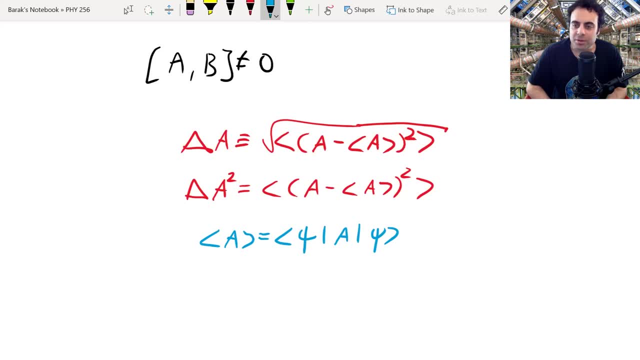 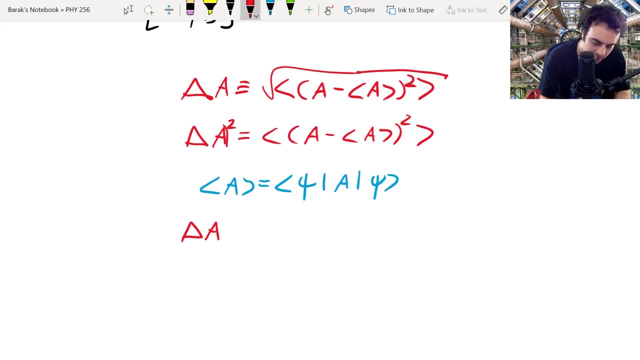 at the moment. So the square of the standard deviation is given by delta a. let's write parentheses just because it's not the standard deviation of a squared, it is the standard deviation of a, and then we square that and there's a difference between the two. 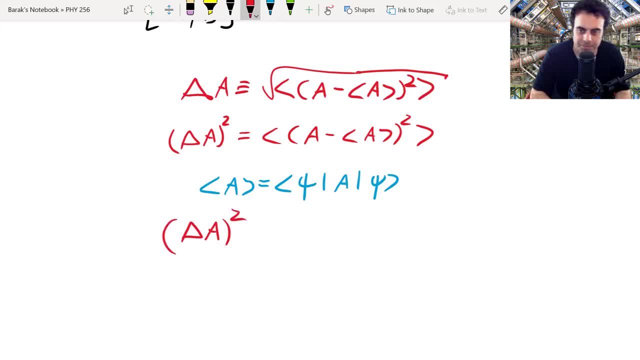 So delta a squared is equal to Psi, a minus expectation value of a squared times Psi. Okay, Now a minus expectation value of a squared is just a minus expectation value of a times itself. So we can write Psi a minus expectation a. 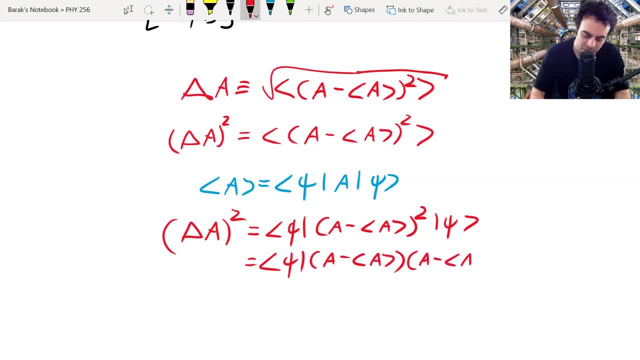 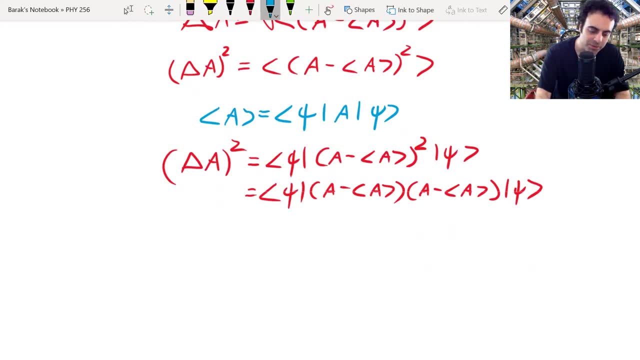 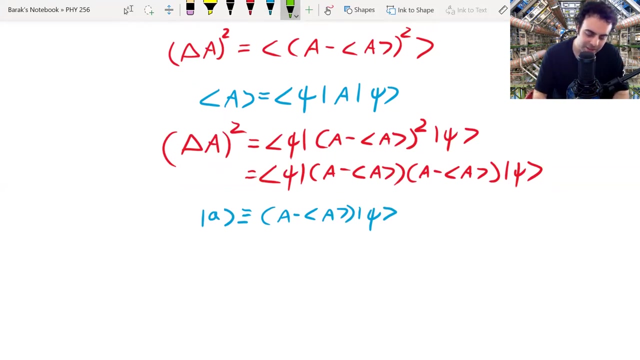 times a minus expectation, a times Psi. And now I'm going to define a new ket: a to be a minus expectation value of a times Psi. And now remember that a is her mission, the operator. a is her mission because it represents an observable. 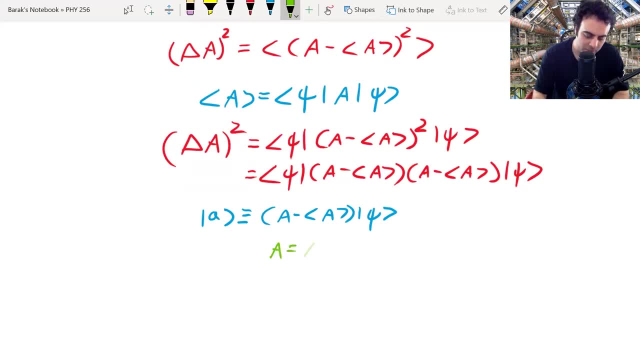 So we have that a equals a dagger, by definition, And of course, the expectation value of a is just a number and it is a real number because, remember, the expectation value of a hermitian operator is always real. So when we take the 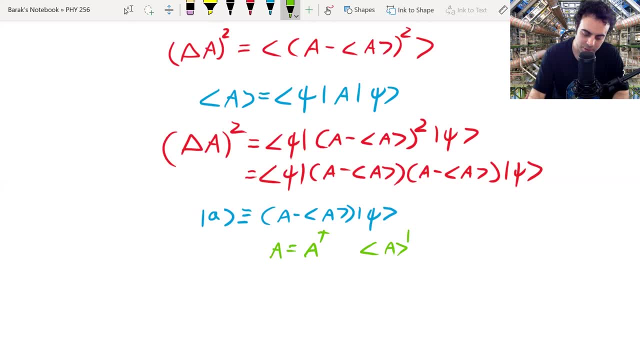 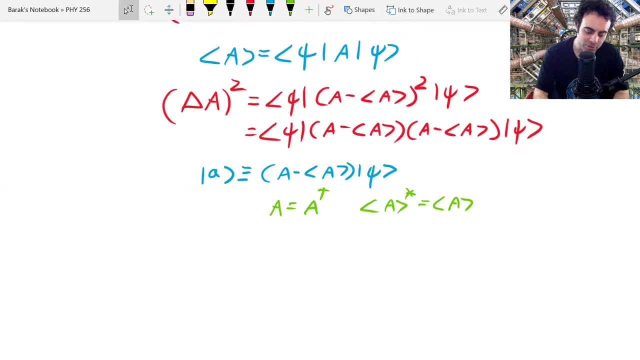 adjoint of that, which is actually the complex conjugate of this number, it is equal to itself. So if I take the adjoint of this whole equation in blue, I'm going to get that bra a. so the adjoint of the ket a. 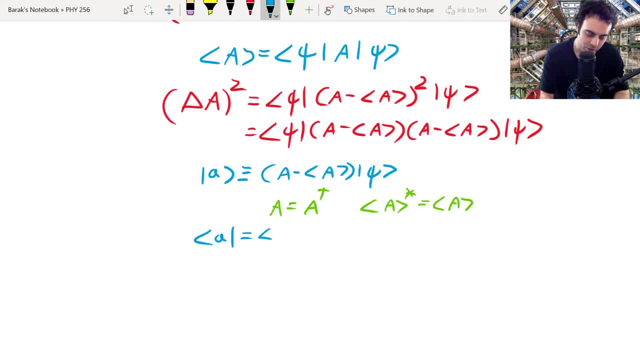 is equal to bra Psi times a minus the expectation value of a. So we took the adjoint of this whole equation, but a and expectation a are both equal to their own adjoint. so this is what we get Therefore. 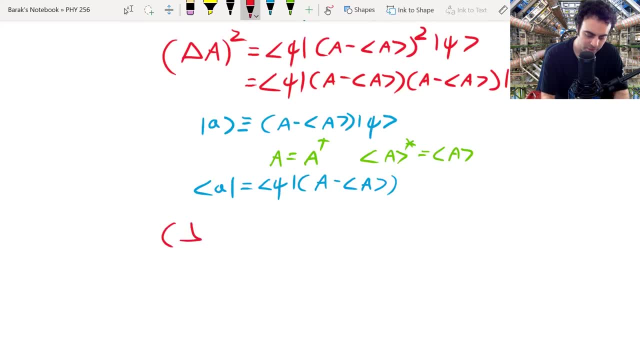 we can simply write that standard deviation of a squared is equal to a. So now, this is a, the lowercase a, and this is also lowercase a, so it's just lowercase a times itself. In other words, it is the norm of the ket a squared. 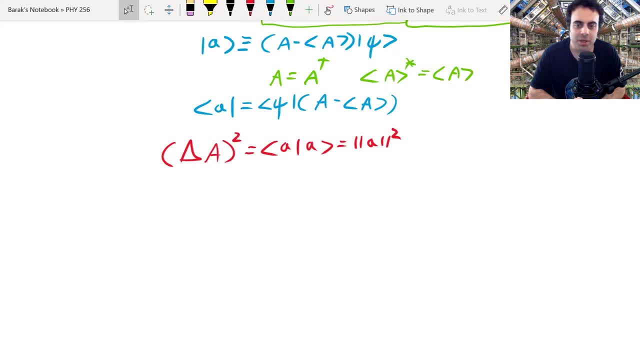 So far we only talked about the hermitian operator a, but we do have another hermitian operator, b. Of course they are both the same kind of operator, so the exact same calculation applies also to b, and we find that. 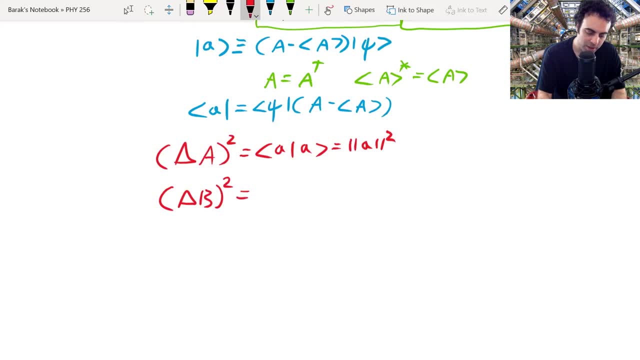 the standard deviation of b squared is equal to some lowercase b ket times itself, or in other words to the norm squared of lowercase b. where lowercase b is just defined in the same way, it's b minus expectation value of b times psi. 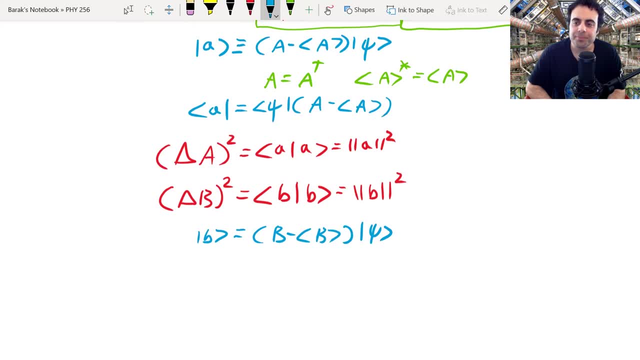 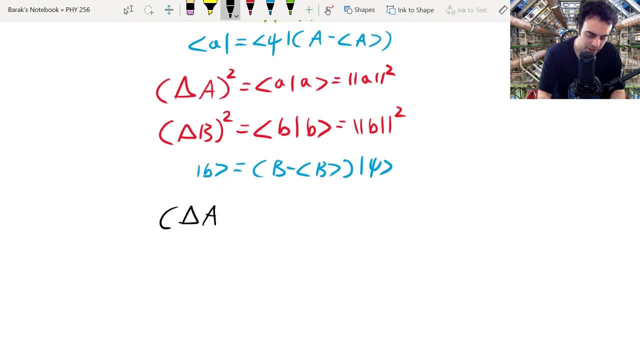 So now comes the most interesting part. So the product delta a squared times delta b squared is equal to norm of a squared times b squared. Now remember the Cauchy-Schwarz inequality that we learned, I think, in the second lecture probably. 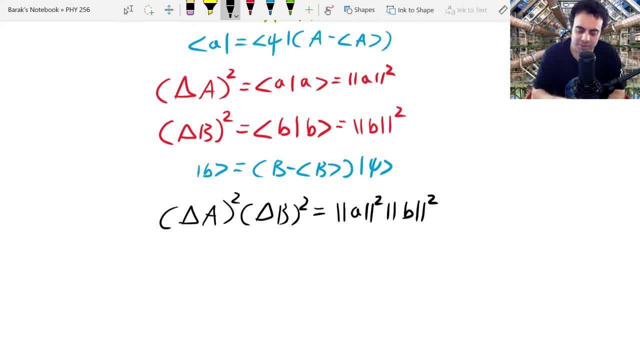 And this Cauchy-Schwarz inequality tells me that the product of the norms of those two vectors is greater than or equal to the magnitude of the inner product between those two vectors. Okay, if you don't remember this, you should check the lecture notes. 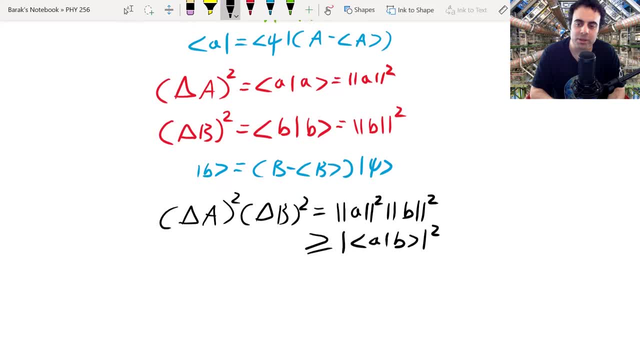 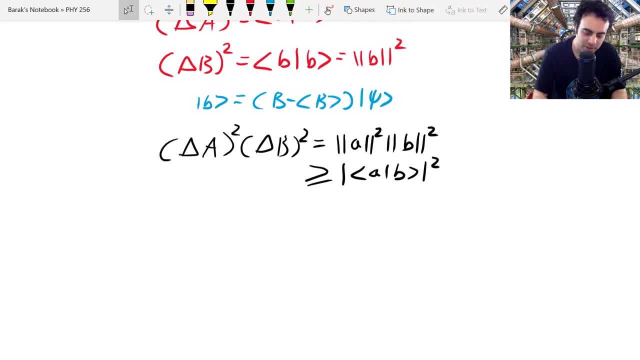 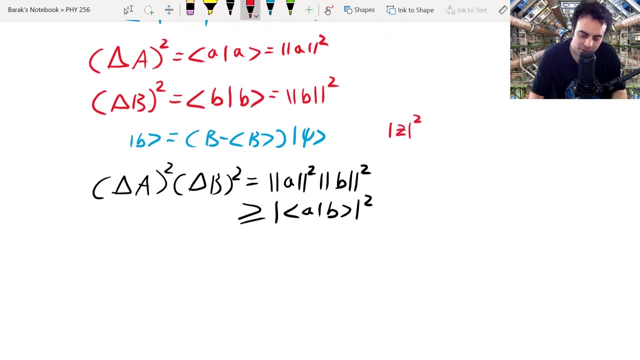 or re-watch the lecture where we talked about it. Okay, so now remember that the magnitude squared- let's say I have z, a complex number- magnitude squared is actually the real value of z squared plus the imaginary value of z squared. 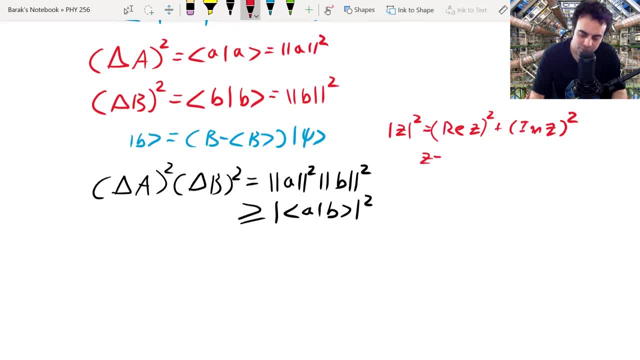 So, for example, if z is equal to a plus ib, where a and b are both real, then z magnitude squared is just equal to a squared plus b squared. Okay, so here it's the same thing, This inner product of a and b. 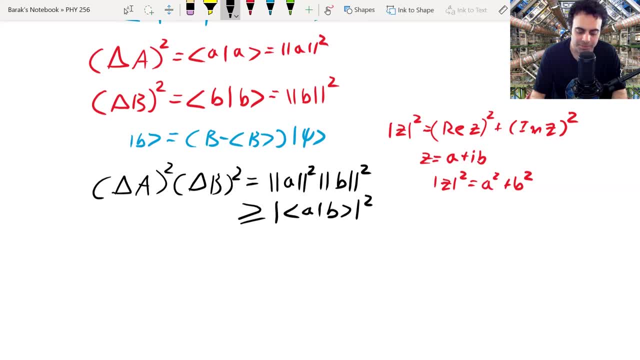 just like any other inner product, is a complex number and therefore I can write that it equals to the real part of a inner product, b squared, plus the imaginary part of a inner product, b squared. Now, this is a sum of two real numbers squared. 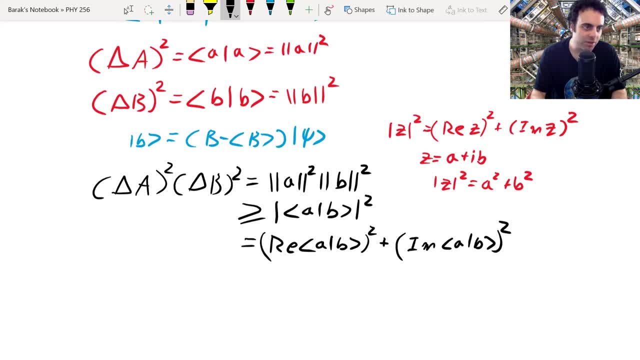 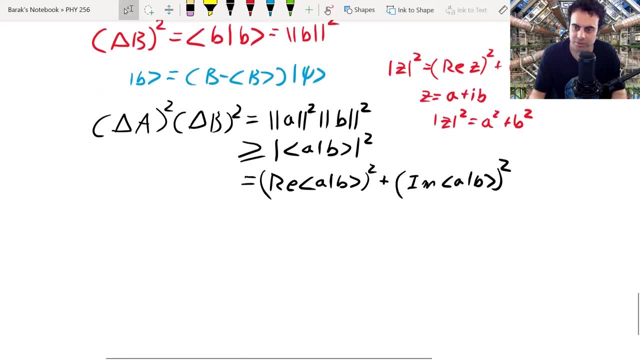 so both of them are positive. If I have a sum of two positive numbers, it is of course larger than just one of the numbers, So we can say that this is greater than or equal to just the imaginary part of a inner product b. 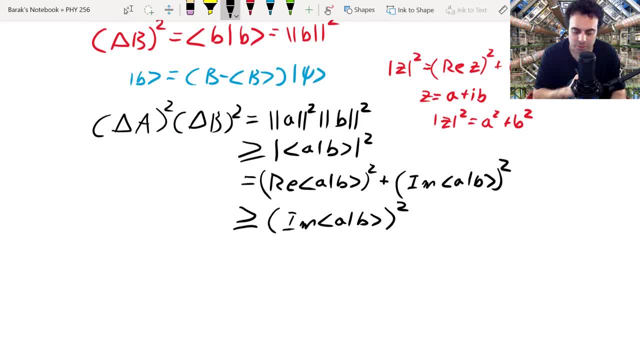 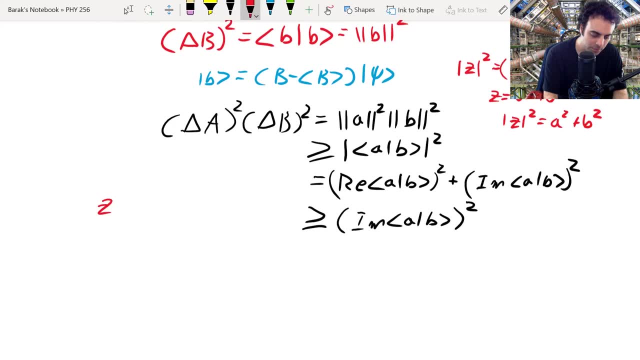 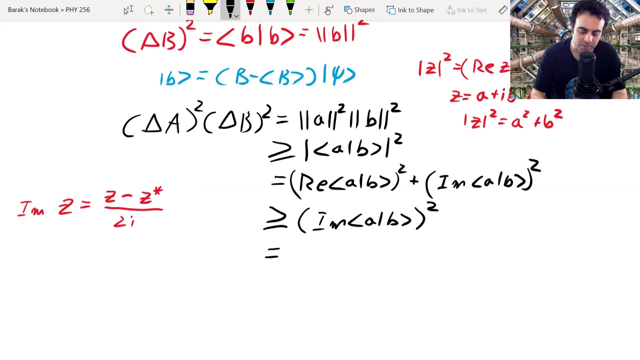 squared. Now also remember for complex numbers that the imaginary part of z is equal to z minus the complex conjugate of z divided by 2i. So the imaginary part is equal to the number a- inner product b minus that number a inner product b. 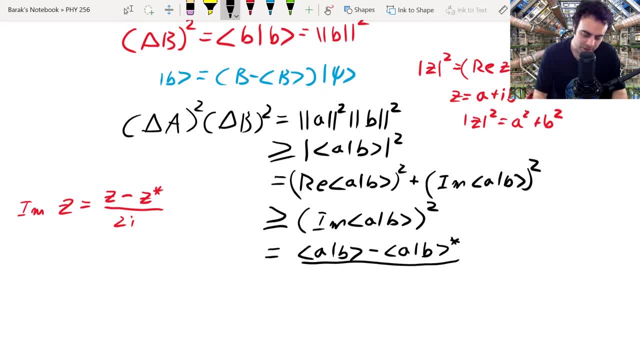 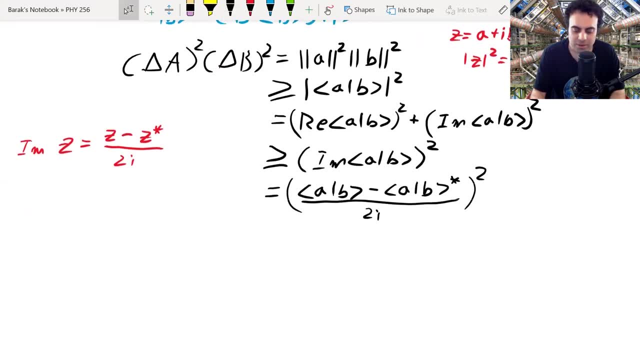 complex conjugate divided by 2i, and all of this squared. Now also remember that if I switch the order of vectors in the inner product, I get the complex conjugate. So this is actually equal to a inner product b minus b inner product a. 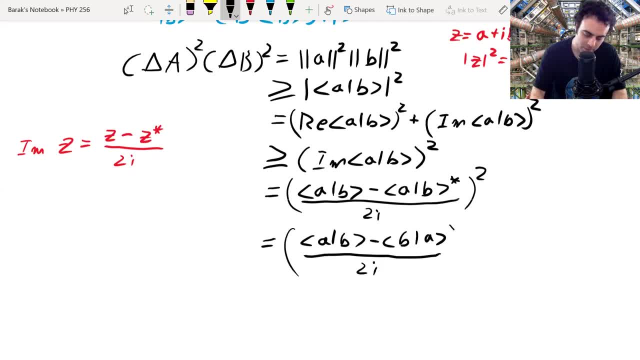 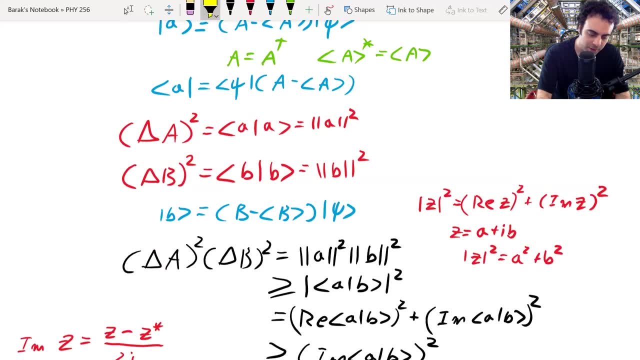 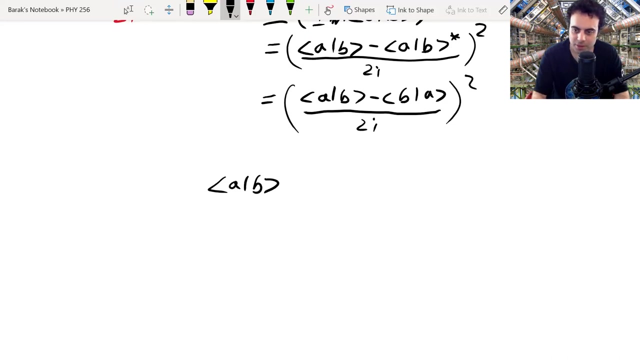 divided by 2i squared. So now remember the definitions of this lower case a and lower case b. So now we're going to actually plug them into this equation. So a inner product b is equal to by definition, so a. 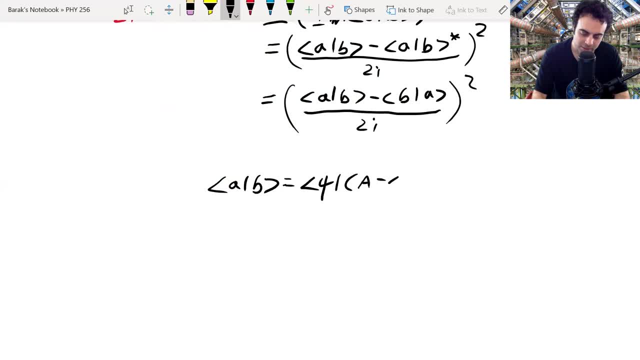 was psi a minus expectation value of a. And then this is times b, which was b minus expectation value of b, times psi. Okay, Let's write it a bit more compactly. So remember we don't actually have to write down the psi's. 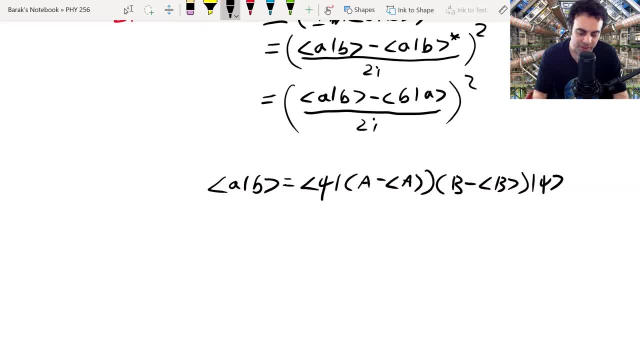 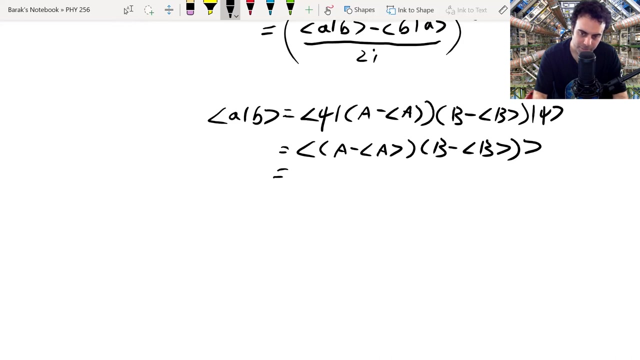 if we know that we're talking about the state psi. So this is just expectation value of a minus a, b minus expectation b. And now we can expand. So this is ab minus a expectation b minus expectation ab plus expectation a, expectation b. 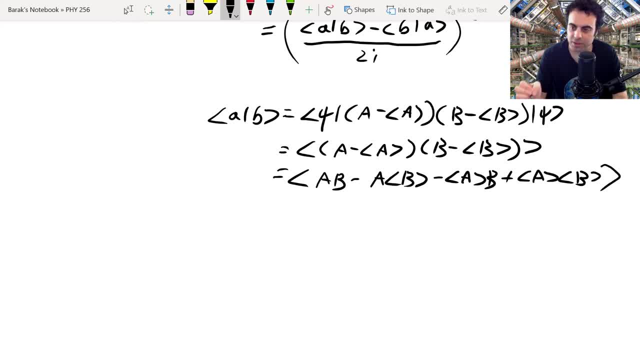 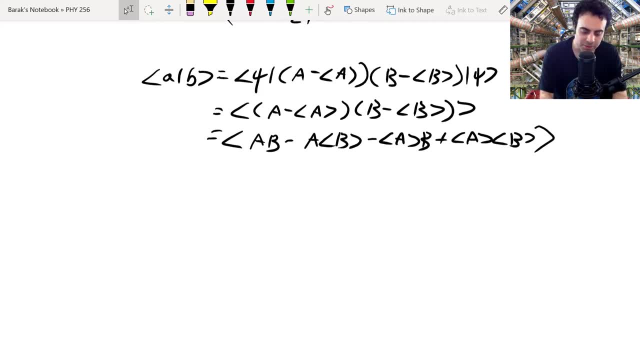 b. all of this inside a big expectation value. the expectation value is linear, so we can just separate this into different expectation values. so this is a b expectation value. and now here the expectation value of a operator times the number. expectation b is just the expectation of a times the number. 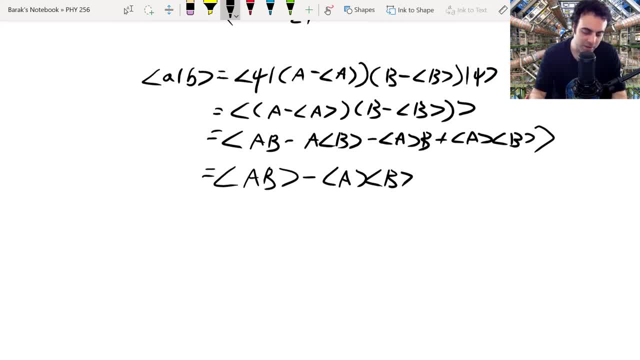 expectation b, because the number just comes out of the expectation value because it's linear. so the second term as well, the number, expectation a, comes out of the big expectation value, and then we're just left with expectation b, and now this is just a number, so it is just equal to itself. 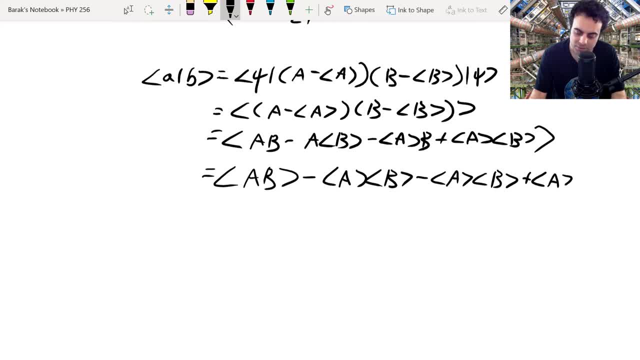 I mean, its expectation is just equal to itself, and now these two last terms over here they actually cancel each other. so we are just left with a b minus a times b. so this was the inner product of lowercase a with lowercase b and similarly the inner product of lowercase b with lowercase a. 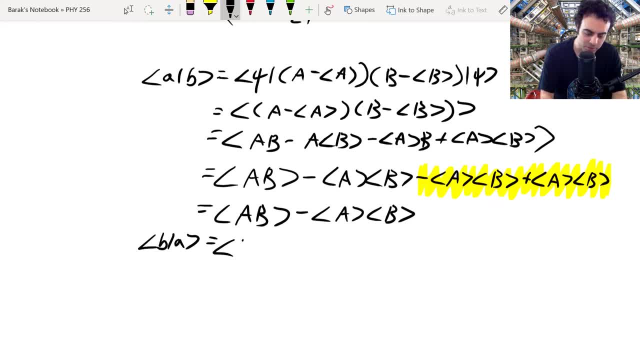 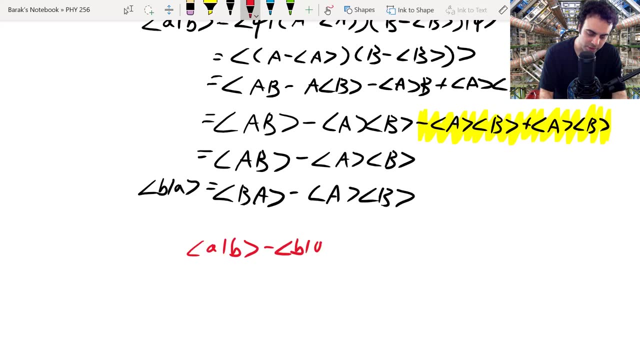 you can do the same calculation and find that it's equal to b a minus a b, which means that a inner product b minus b inner product a, which means that a inner product b minus b inner product a is equal to: so it's this minus this. 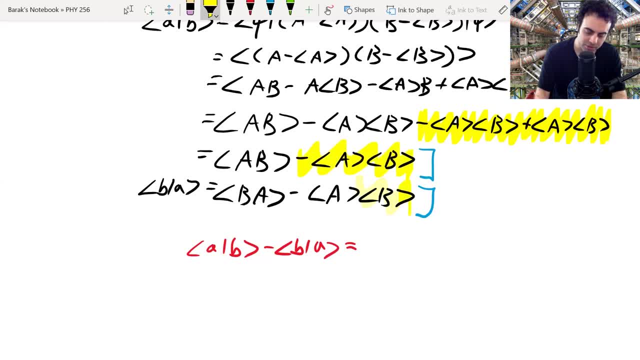 but notice that these two terms are the same, so they cancel each other. so we are just left with a- b expectation value, minus b- a expectation value, which is the expectation value of the commutator of a- b, which is the expectation value of b, which is the expectation value of a- b. 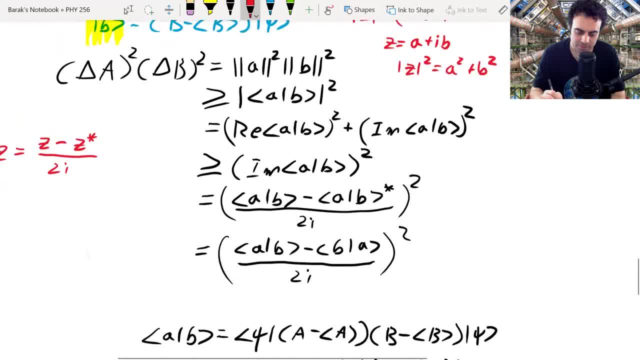 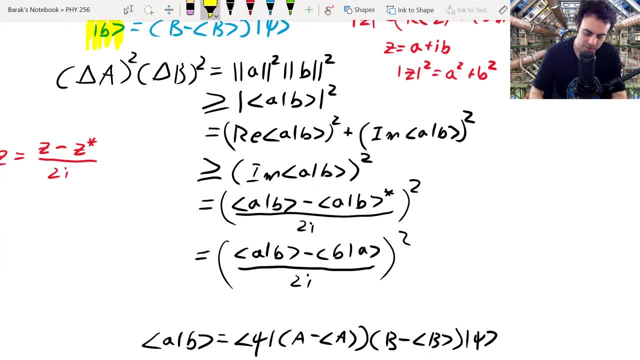 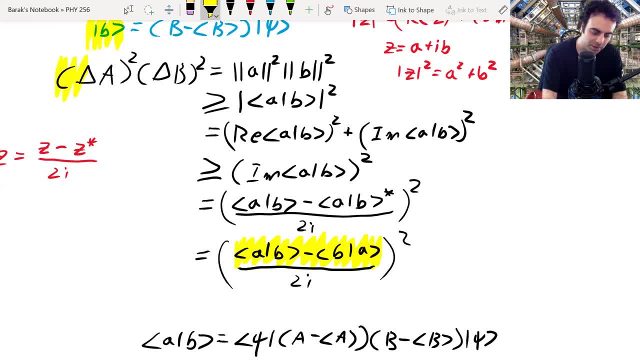 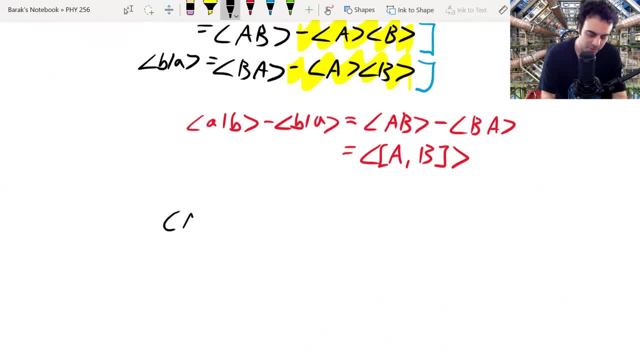 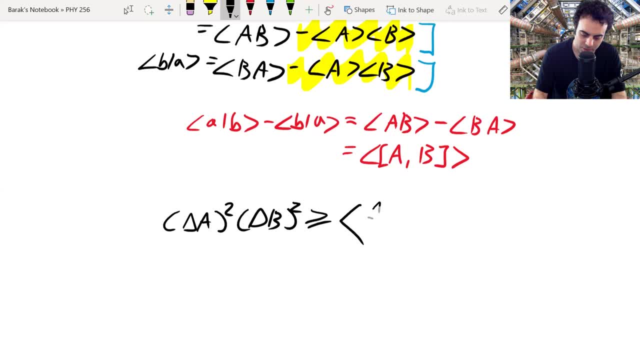 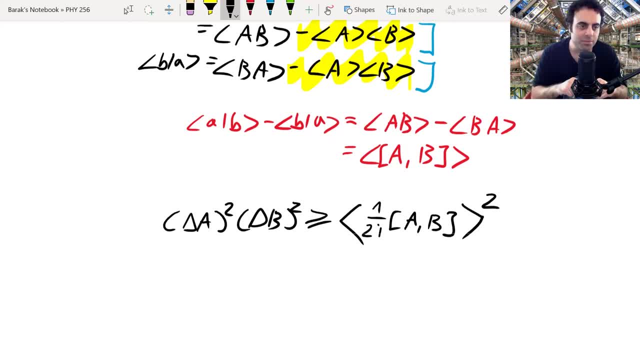 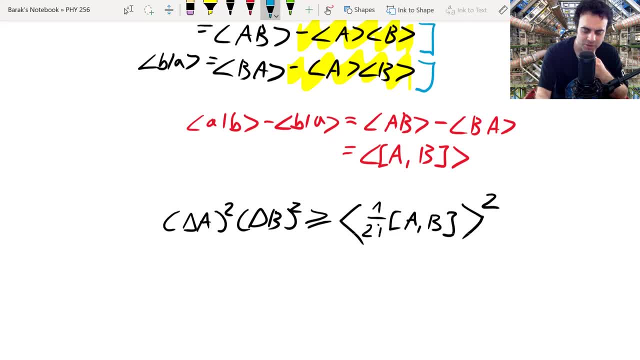 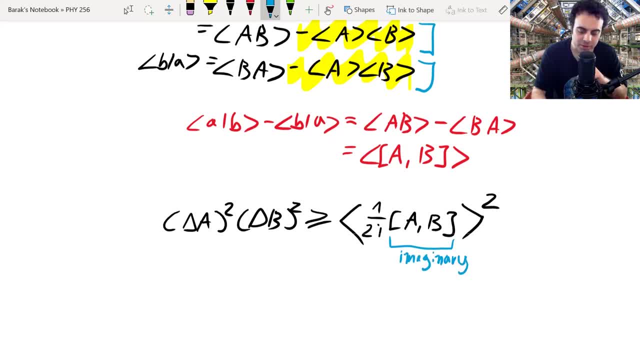 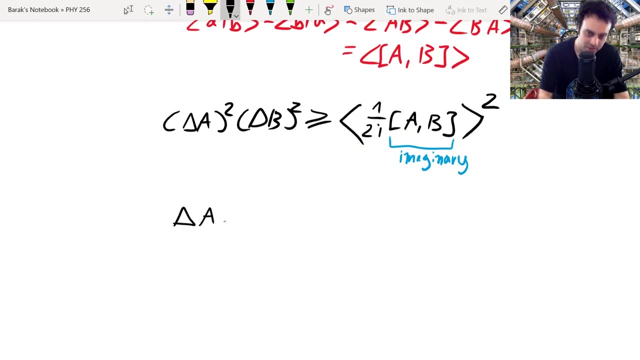 which is the expectation value of a, b, i times the commutator, is actually a real number, because the imaginary number divided by i is a real number. so we can take the square root of both sides and we get finally that delta a times delta b is greater than or equal to one half times the absolute value of the expectation value. 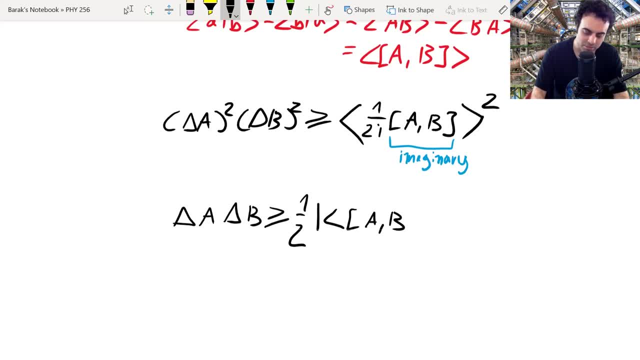 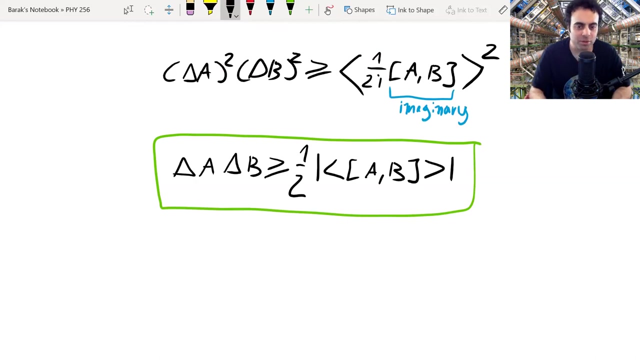 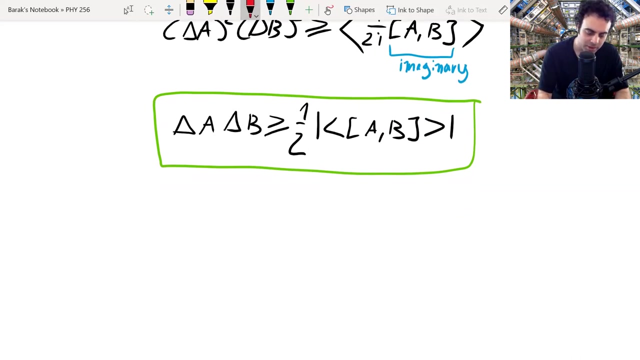 of the commutator of a- b, and this is a very important relation and this is the proof of the uncertainty principle. let's do a quick example. let's say that a and b are position and momentum, and position and momentum we will learn later. they have the following commutator, so x commutator p is just equal to i and, of course, 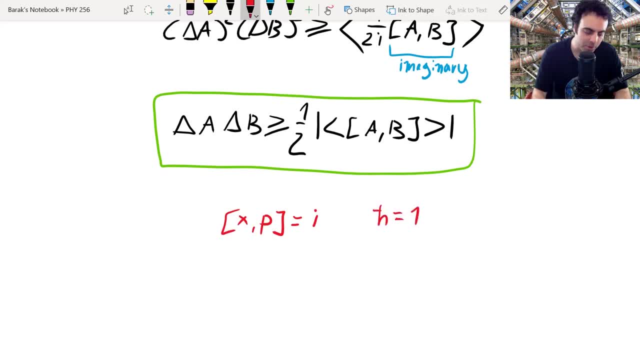 this is in units where h bar equals one. if not, then it's equal to i times h bar, and if i plug it in, i will find that delta x, delta p is greater than or equal to one half times the absolute value of i, which is just one. 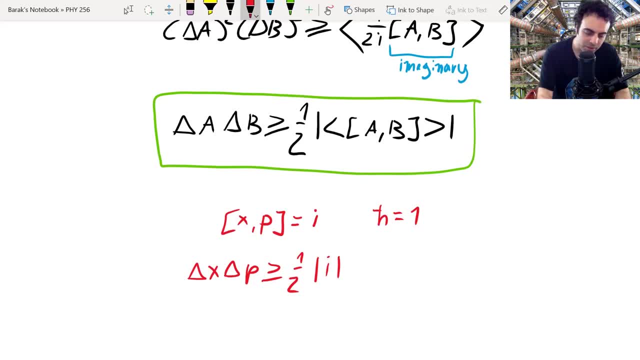 so delta x, delta p is greater than or equal to one half, which is indeed the position momentum- uncertainty relation. i have a question on the chat: is it important to memorize this proof? no, you don't have to memorize any proof. this proof is just because i wanted to show you. 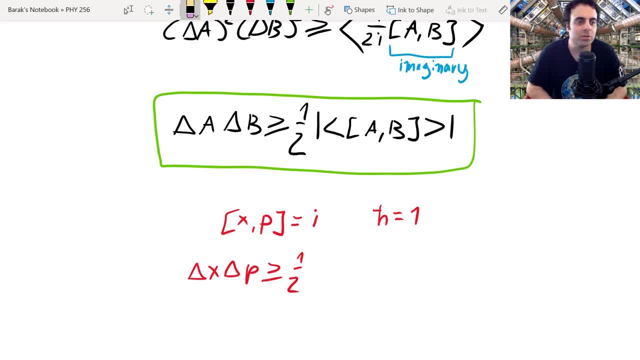 that you can actually derive the uncertainty principle. usually in most quantum mechanics courses, at least in introductory courses, you- just you- can derive the uncertainty principle, get it as a given. it's presented as an assumption and that's not true. it is actually not an axiom. it follows from the axioms of quantum mechanics that we wrote down and we can prove it, and 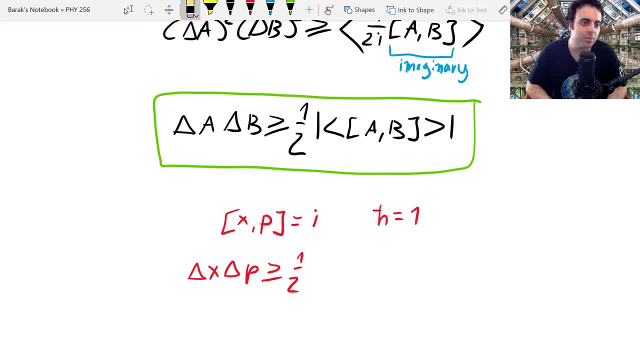 it is a bit of a lengthy proof but it's actually a pretty simple proof so you don't need to memorize it. there's no reason to memorize it in general, all for the purpose of the exam. but definitely you should go over the proof because the proof uses a lot of things that. 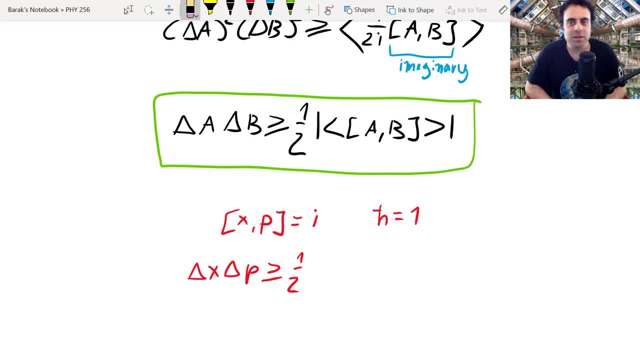 we learned that are important in this course, like inner products and standard deviation and so on. so definitely try to understand how this proof works, but you don't need to memorize it. so i have a question at the end, why can we add one over two i to the inequality? we don't add it. 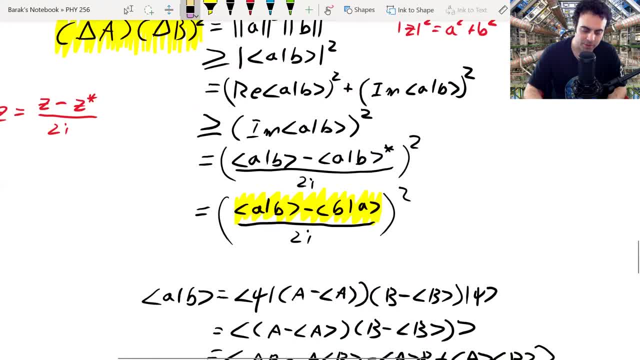 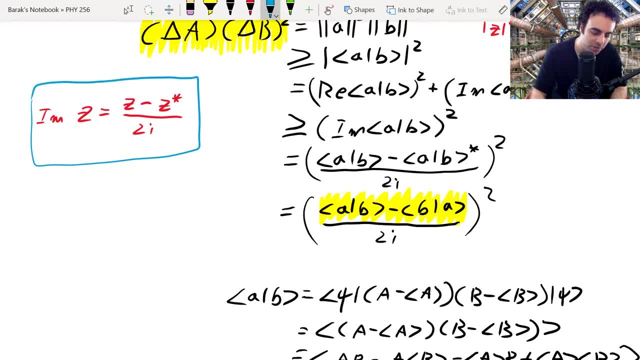 the one over two. i is here because the definition of the imaginary part of z is z minus conjugate z over two i. so here we have the imaginary part of a in a product b. it is equal to a in a product b minus its conjugate divided by two i. so it was there all along. 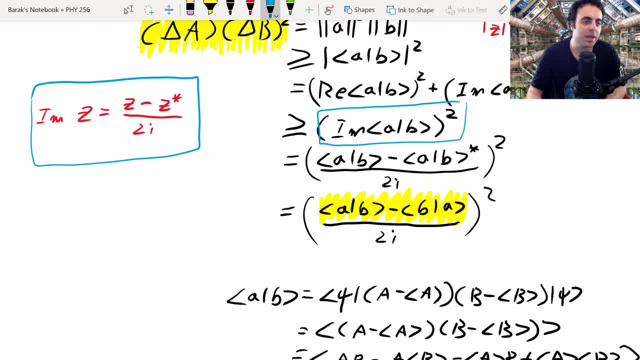 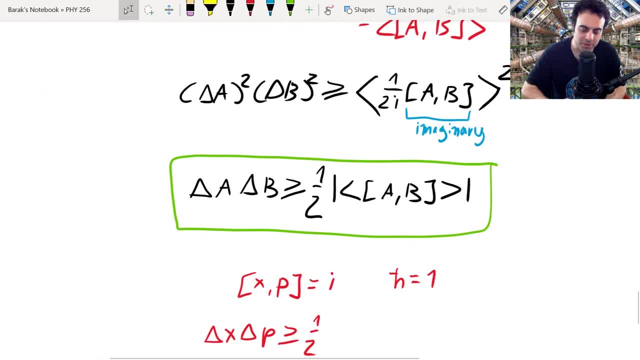 so i have a question on the chat. so that relationship at the end is basically the uncertainty principle. yeah, this relationship in green is the general uncertainty principle. that applies to any two operators, a and b, that are Hermitian operators, of course. if they commute, then you get that delta a, delta b is greater than or equal to zero, which it has to be because they're. 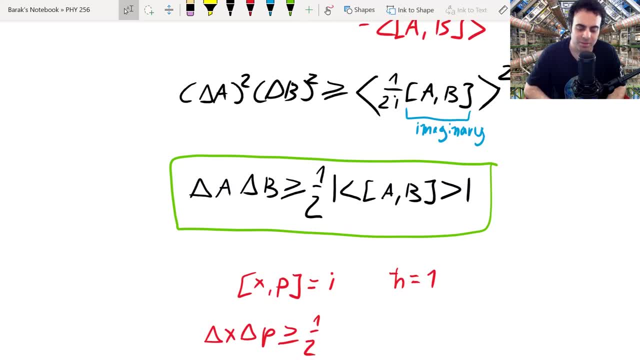 both non-negative numbers. so if the two operators commute, then this is just trivial, but if they don't commute, then you get this relationship. i have another question. the question on the chat is: would you not be able to get an even stronger principle if you let the real part in instead of ignoring it? sure, i mean. 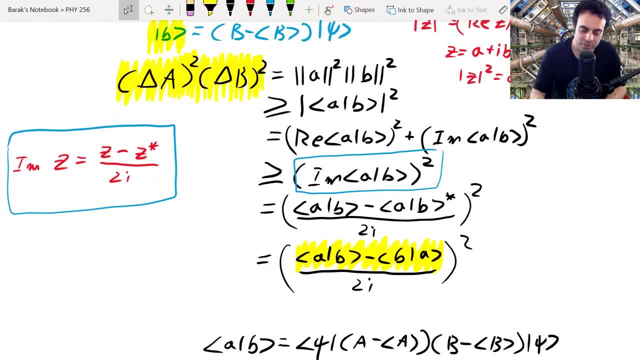 this is here. we just we do two things actually, those two inequalities we're using. the first inequality is the Cauchy-Schwarz inequality and the second inequality is just that we take the real part out. so technically, yes, if we left the real part here, then we would get an even stronger uncertainty principle, but also it wouldn't. 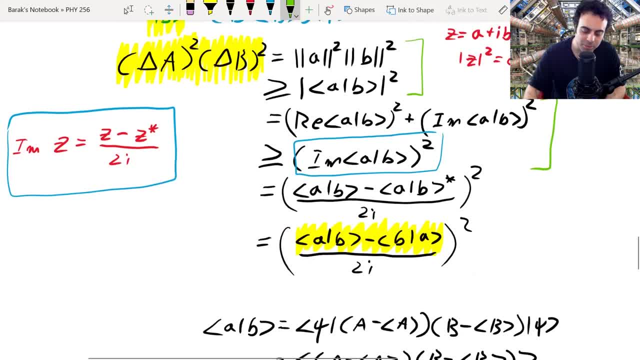 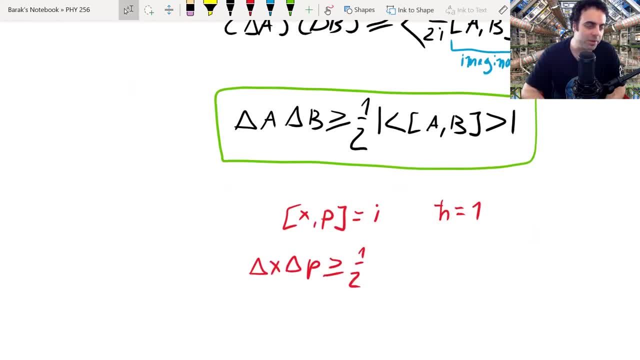 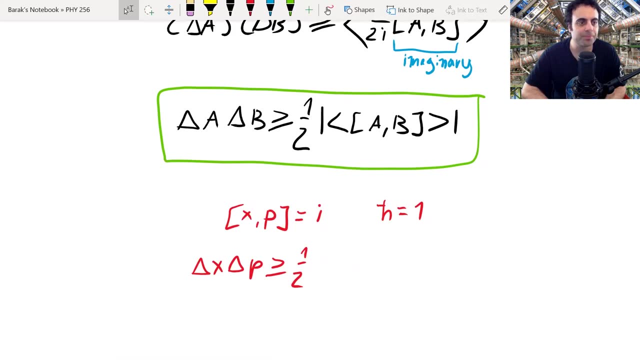 be, it wouldn't have the simple expression that we got here. it will be a much more complicated expression, so theoretically you could do that, but there's no need to. this is the relationship that we usually use in either a tutorial or a homework. you will get to calculate the uncertainty relation for 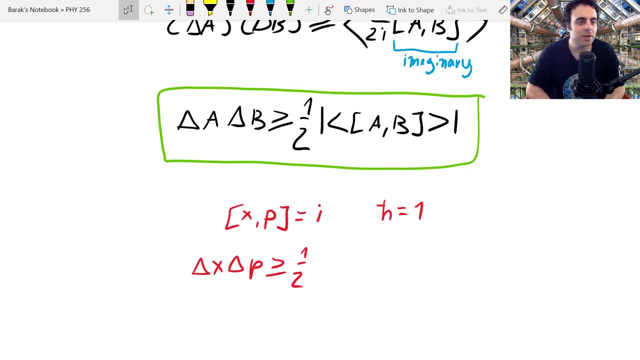 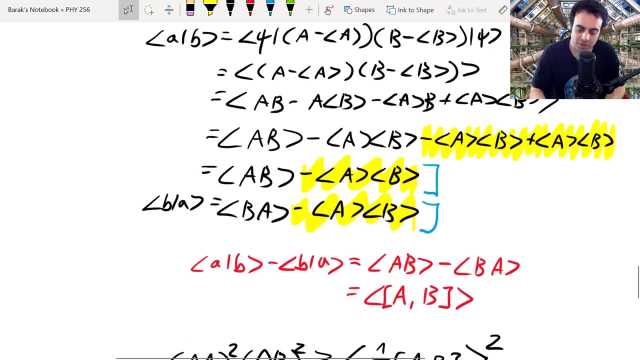 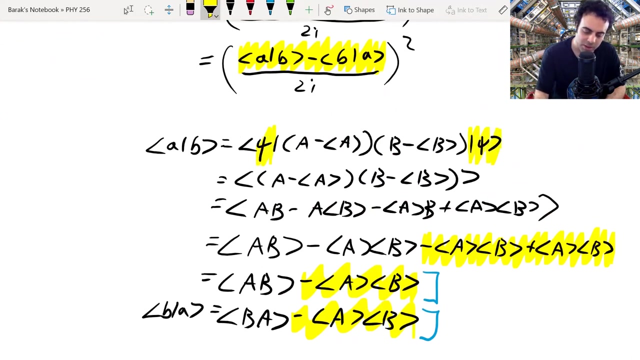 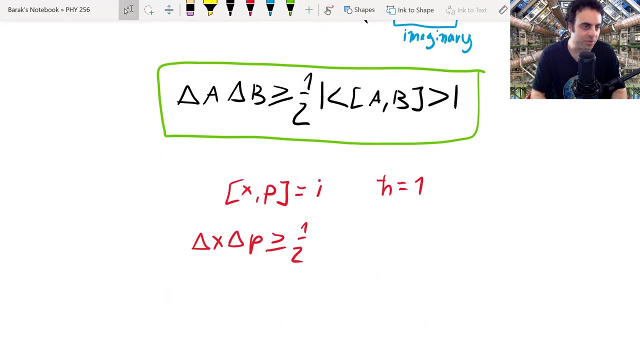 the two Pauli matrices, sigma x and sigma y, and then you'll see that there is an uncertainty relation, not just for position momentum but also, for example, for spins. also another thing i need to tell you is that here we used this state, psi, to do the calculation, and in the case of x and p the result is independent of psi.